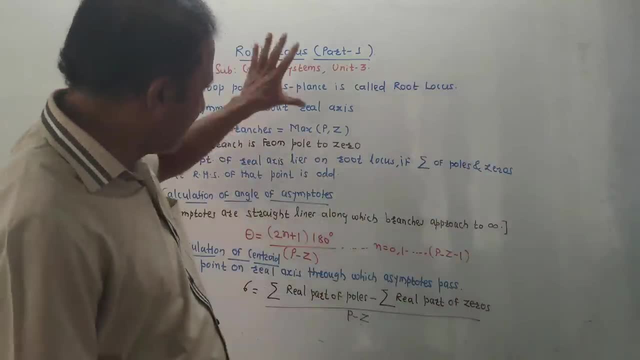 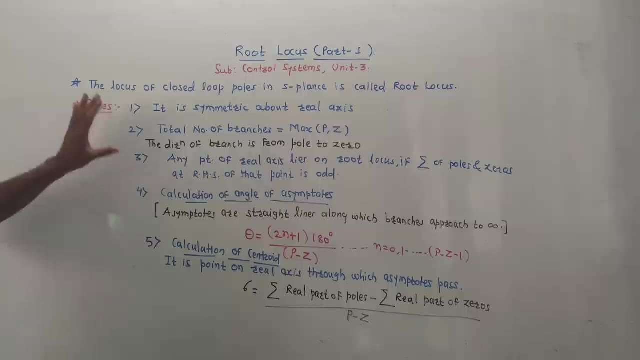 graph paper. For bode plots we need semi-lock papers, but this should be drawn on the normal graph papers. So, without wasting the time, let us start studying what are the rules which are applicable. These rules will be a little tough for you, but while solving numericals, I will be 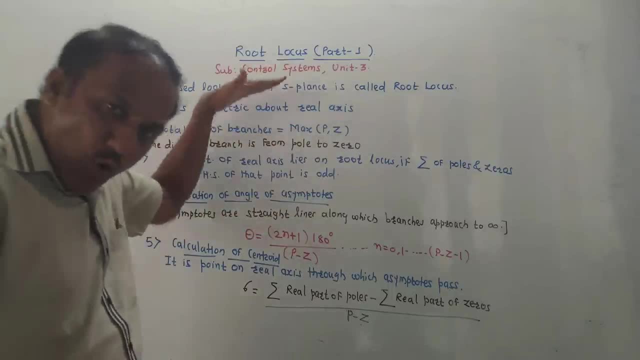 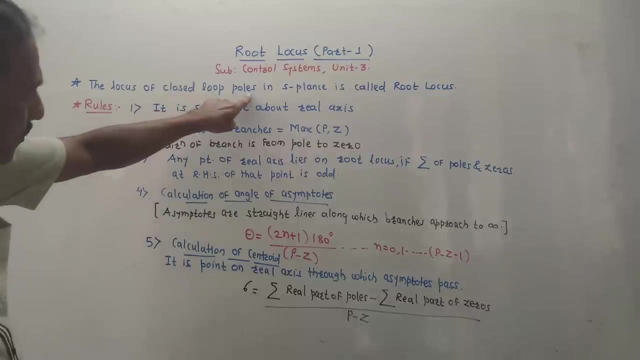 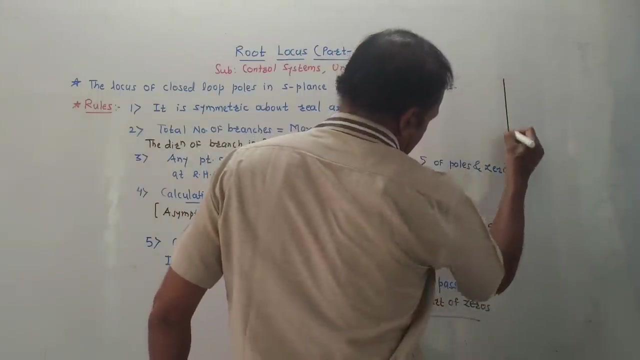 explaining every rule in detail. Just, we are taking overview of each rule. First rule is before that: what is the root locus? It is locus of closed loop poles in S plane and it is called the root locus. What does S plane mean? S means Laplace. On this axis, on X axis, we write real part of S. S means 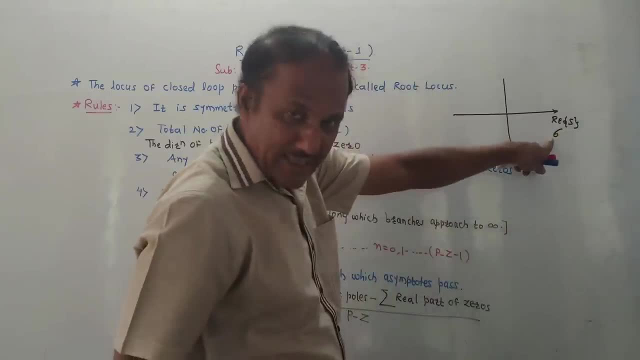 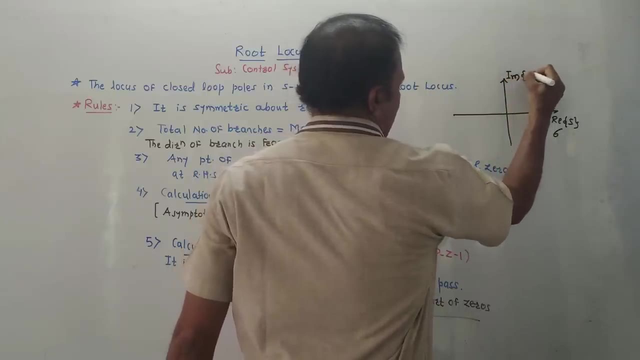 Laplace. This is denoted by sigma. Real part of S is sigma. It is plotted on X axis, whereas on Y axis we are supposed to plot the imaginary part of S. S is Laplace and it is also denoted by sigma. 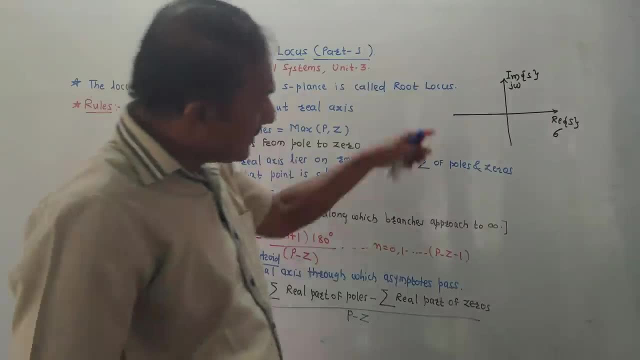 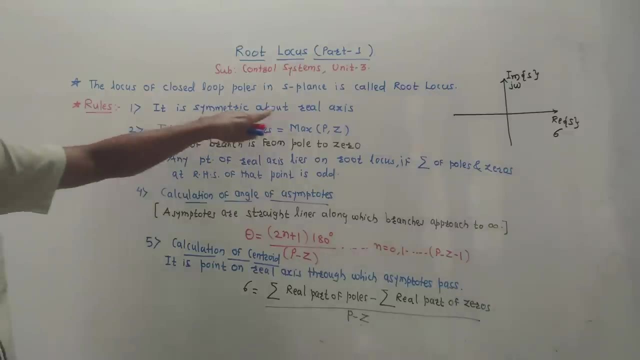 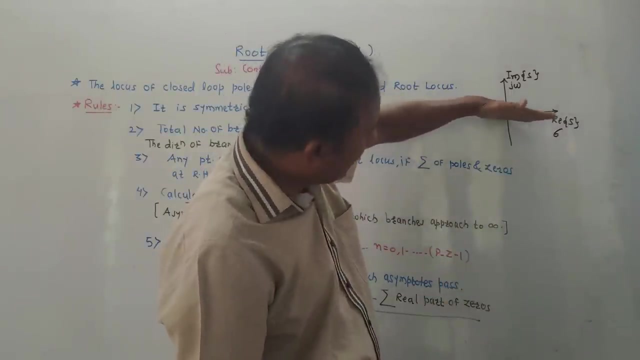 It is also denoted by j omega. So it is graph of sigma versus j omega. This is called S plane. Then first rule is: it is symmetric about real axis. Which means, whatever graph we plot should be symmetric about real axis. Real axis is this: It should be symmetric about real axis. Second rule: 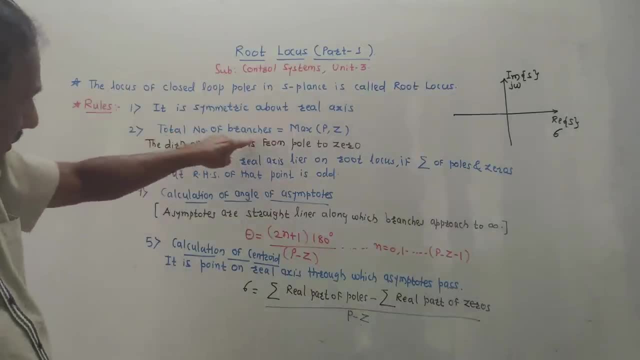 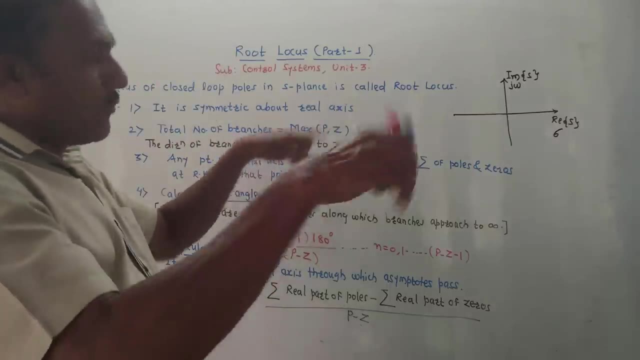 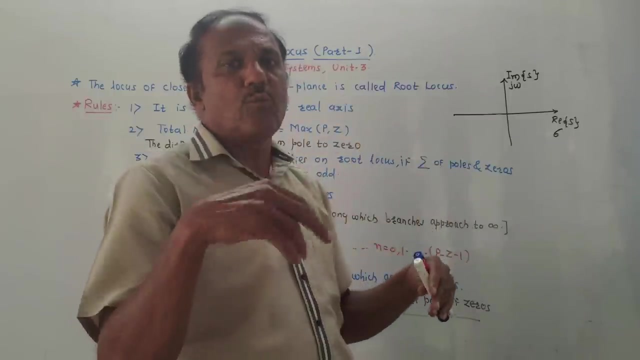 total number of branches means how many branches should be there in root locus. That is equal to zeroes. Z means zeroes. We have already studied. There is an equation in which there is numerator term and denominator term, So the roots of numerator are called zeroes, Roots of denominator. 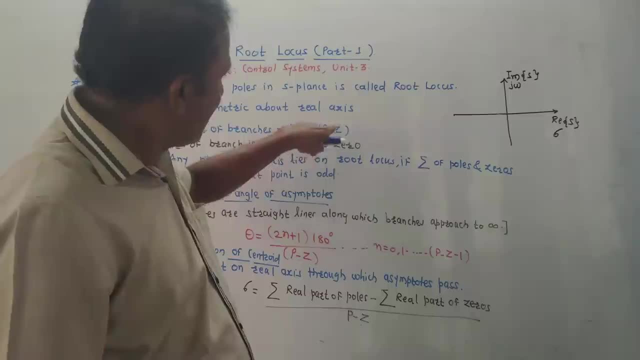 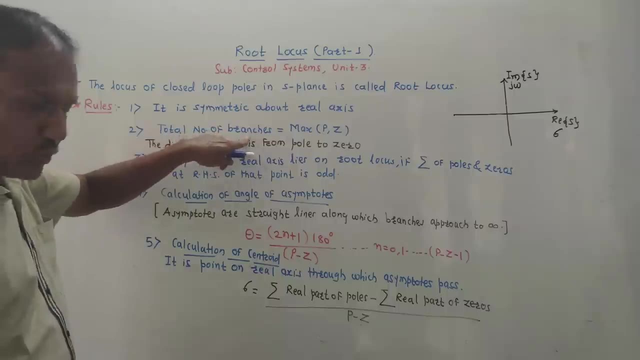 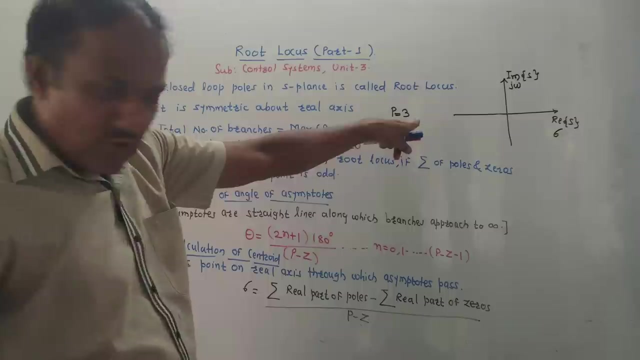 are called poles. So P represents number of poles, Z represents number of zeroes. The maximum value in that will represent how many branches will be there in root locus. For example, in any calculation poles are 3 and zeroes are 2.. So its maximum value is 3.. Out of 2, 0. 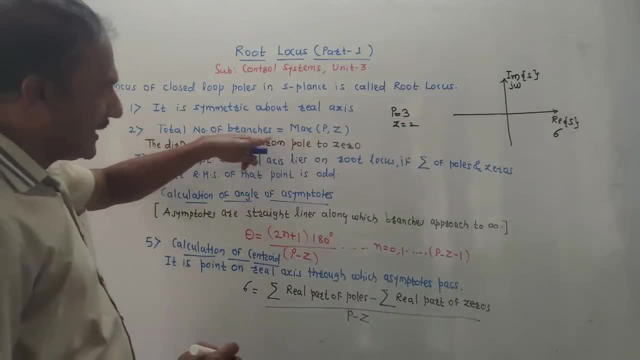 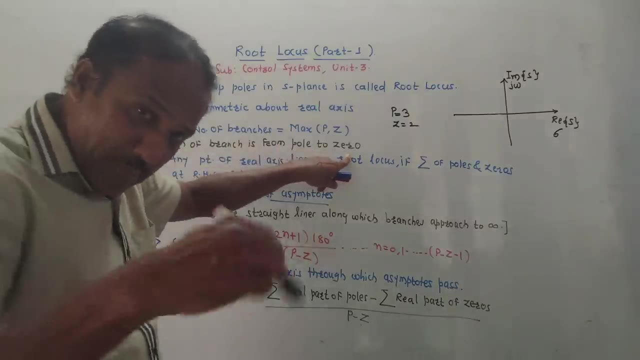 will be 3.. So there will be 3 total number of branches for the root locus. The direction of branch, direction of every branch is from pole to zero. Means every branch will start from pole position and end at zero. So it is from pole to zero. Third rule: any point. 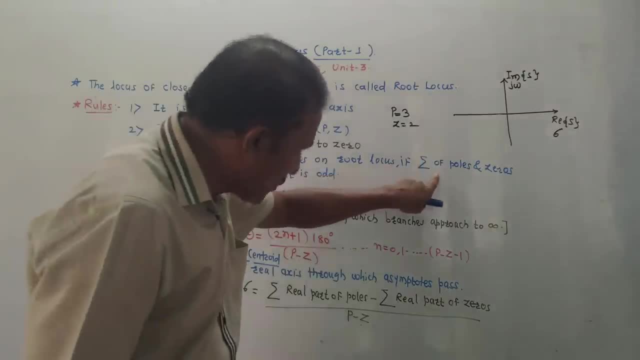 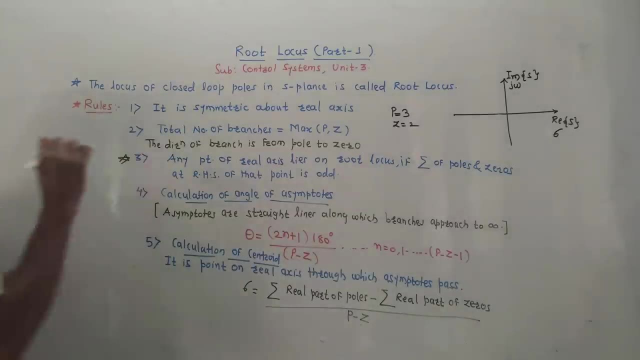 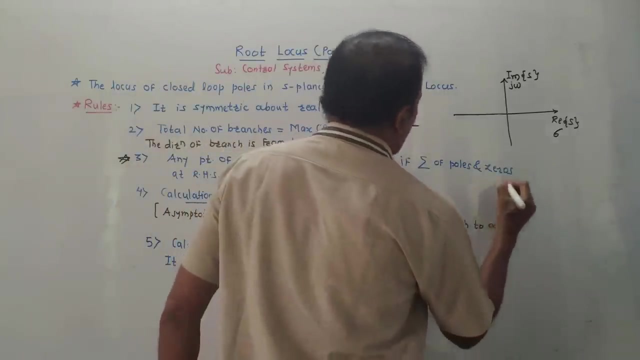 on real axis lies on root locus. if summation of poles and zeroes at the arhs of that point is odd, This is the most important point. See what does this mean? This means that suppose we have calculated poles and zeroes of any numerical. Now remember one concept. 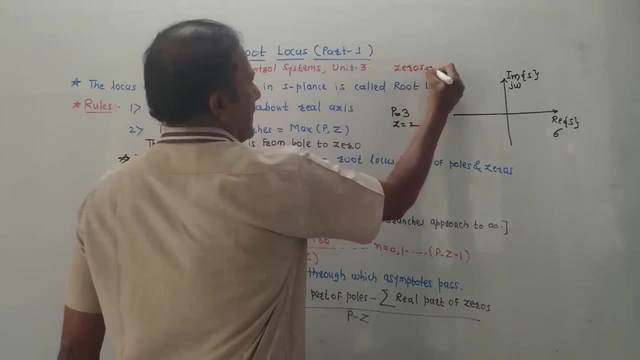 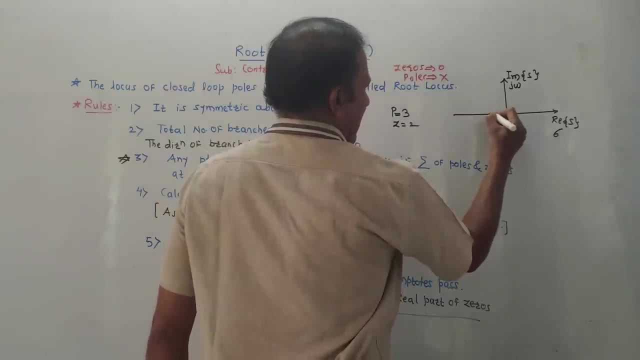 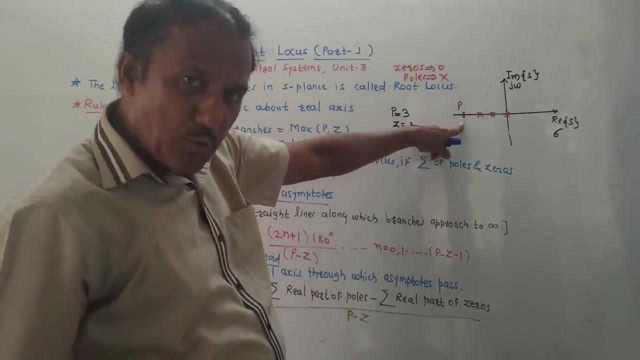 the zeroes. that is denoted by small circle, poles, that is denoted by notation cross. So suppose a diagram is like this: Here is a zero and here is a pole, And this point is suppose P. I have to check point P. Is it part of root locus or not? How to think On? 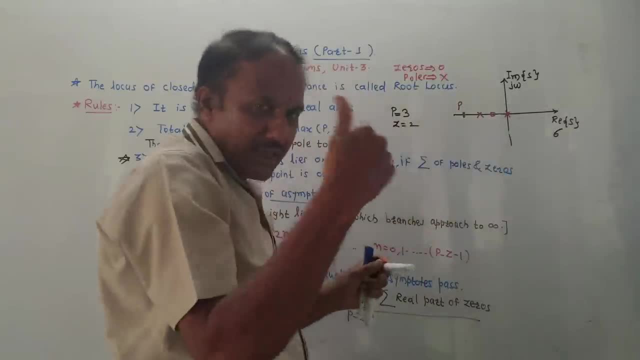 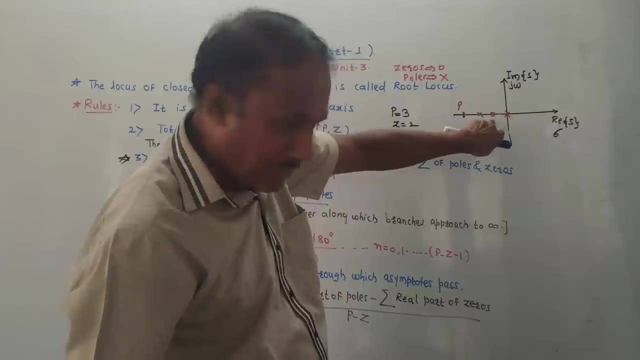 the right hand side of point P means here Are there poles or zeroes. That is important. How many poles and zeroes are there? 1,, 2, 3.. Actually there are 2 poles and 1 zero. This centre part is zero. This is pole, this is another pole. So 2 poles and 1 zero means 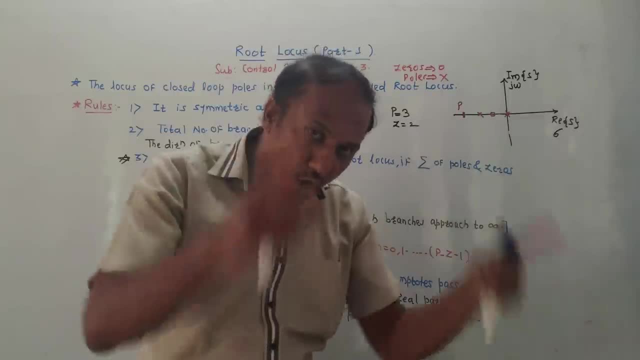 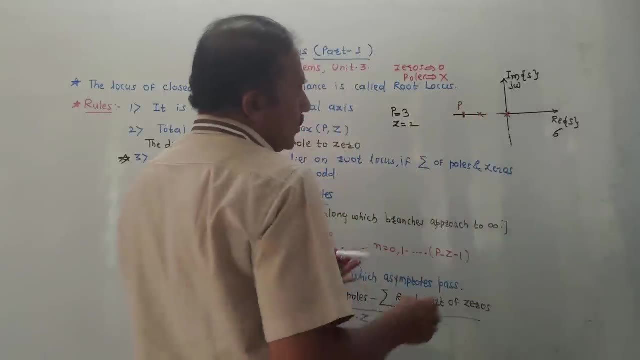 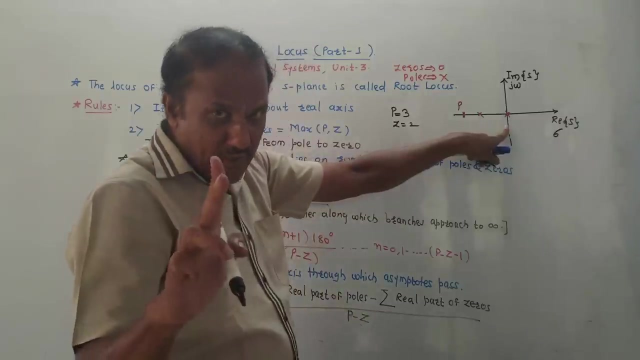 total number of poles and zeroes are 3.. 3 number is an odd number, So point P is part of root locus. Suppose I remove 0 from here and there are only 2 poles. So at the right hand side of point P there are 2 poles, Means here number 2 is there. 2 is even number. So what? 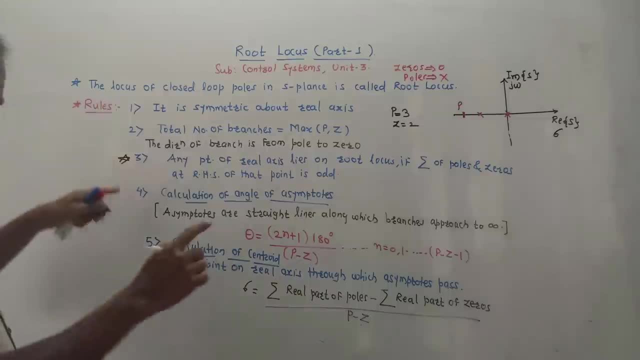 is your point P? A point P is not the part of root locus. likewise, As I have told you, this rule will become clear to you while solving numerical. Next is calculation of angel and asymptote. Basically, what the meaning of this term asymptote is, I have written the definition. 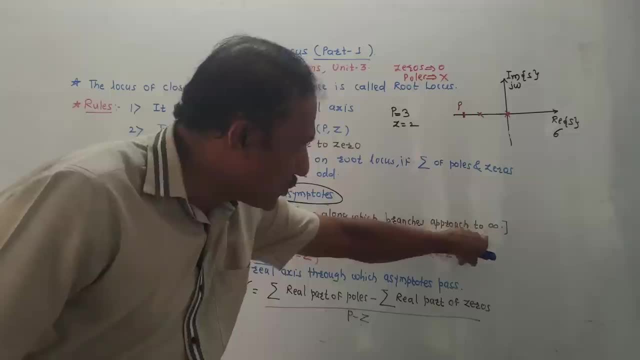 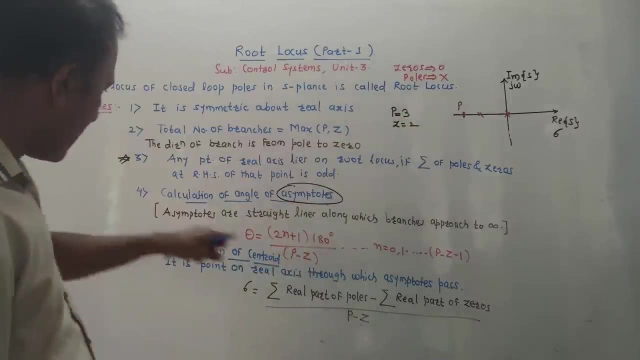 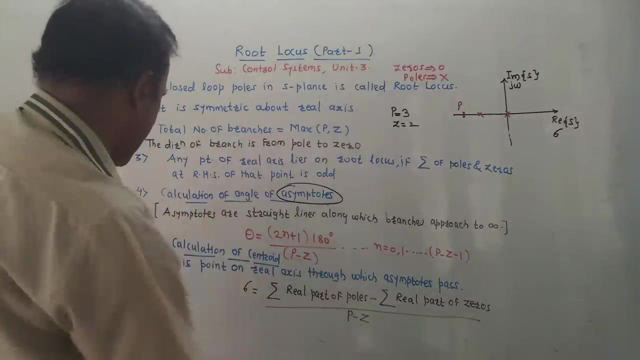 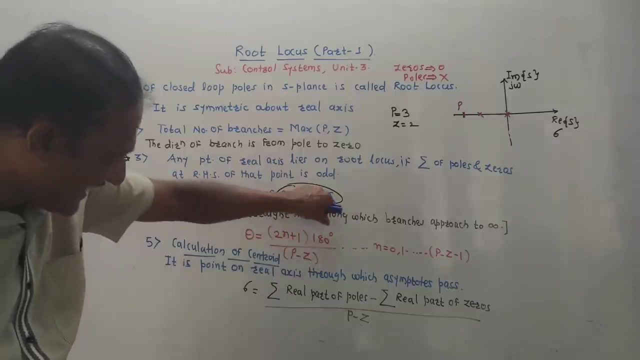 down this too. Asymptote are straight lines along which branches approach to infinity, Which means some branches of root locus. they approach towards infinity, they go towards infinity, those which are moving towards infinity. and how to calculate the angle of this formula? to calculate the angle 2n plus 1 into 180 degree. this is for degree. 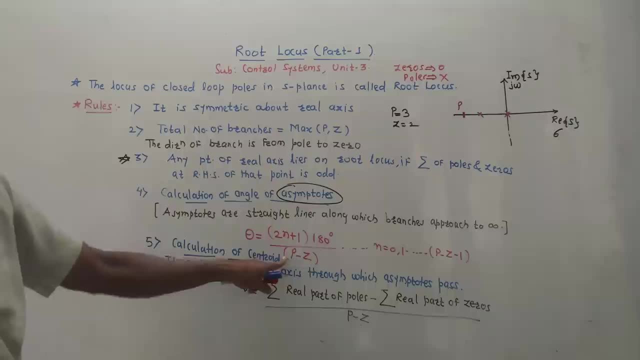 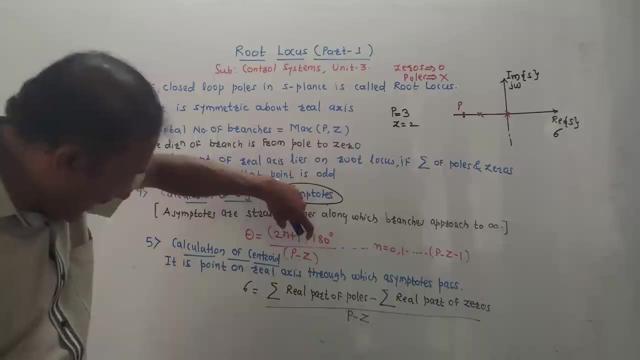 180 degree, divided by P minus Z. as usual, P means number of poles, Z means number of zeros. theta is angle made by asymptotes. now we have to put the value in the formula and solve it, and it has n variable. its range is 0, 1, 2, 3, up to P. 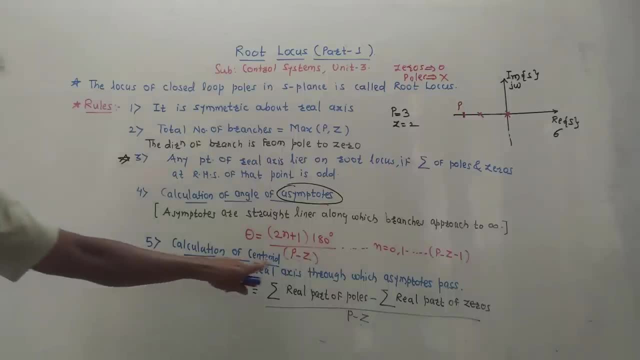 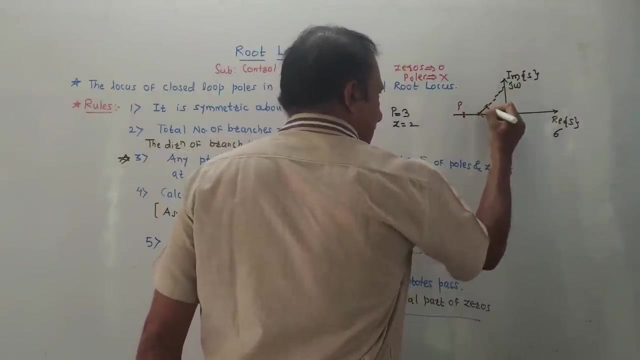 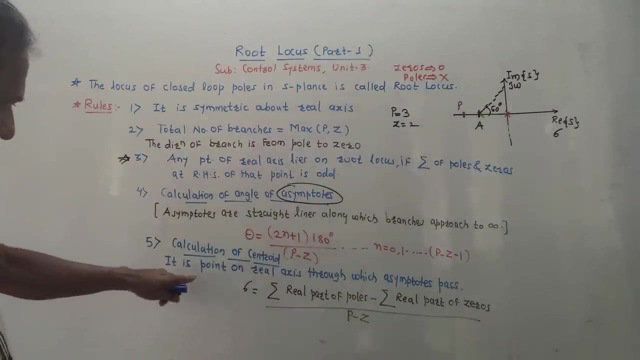 minus Z minus 1. fifth rule is calculation of centroid. centroid will be trawing angle a spilled over P, that is, P a hé pass alright. so this is called the centroid. This is the formula to calculate. centroid is denoted by Sigma. It is summation. this symbol is of summation, Summation, real part. 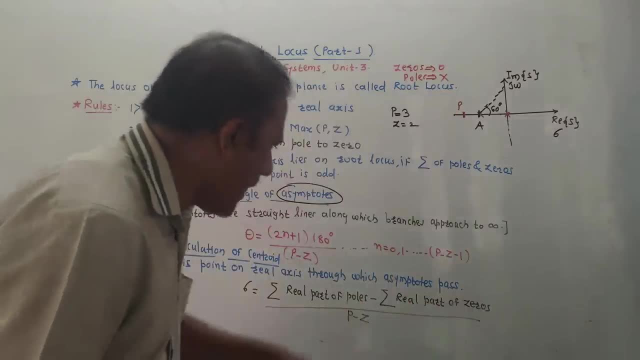 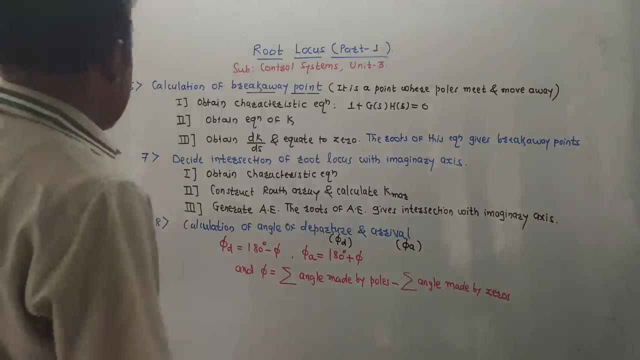 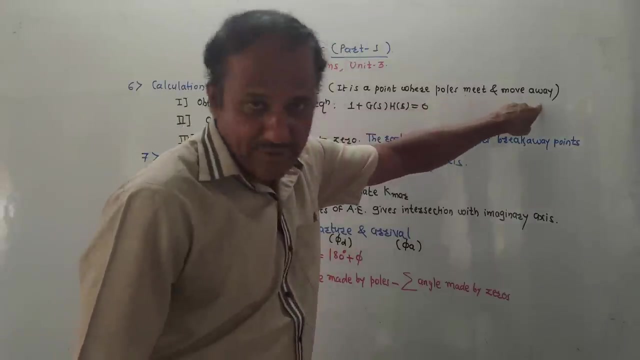 of poles minus summation real parts of zeros upon p minus z. As usual, p means number of poles, z means number of zeros. Next rule, rule number 6: calculation of breakaway point. Now, what is breakaway point? It is the point where poles meet and move away. Means poles. 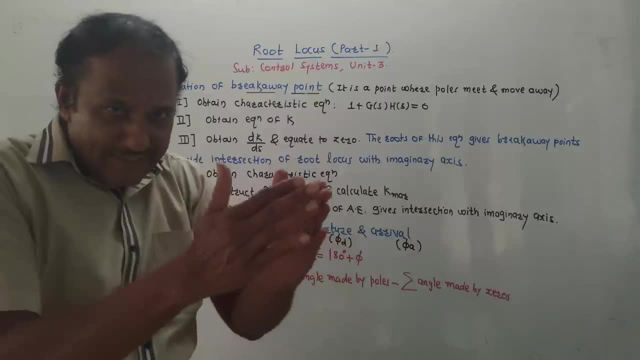 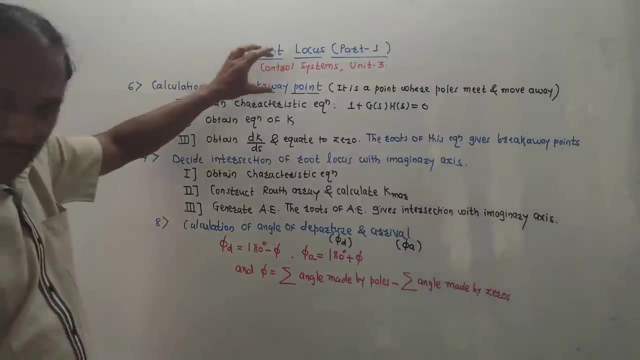 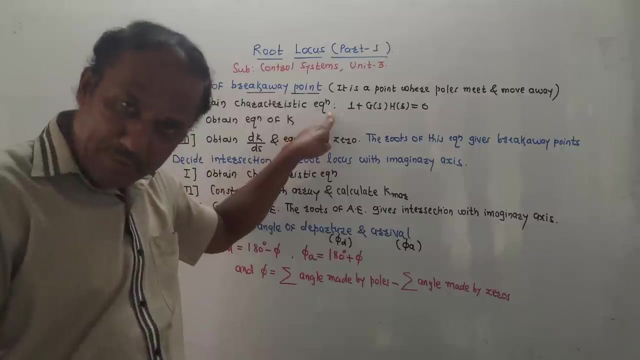 collide at one particular point and then they get splitted away. So this point is where the poles meet and move away. that is called breakaway point. How to calculate it? I have written its steps. First step is to obtain characteristic equation. We know how to obtain. 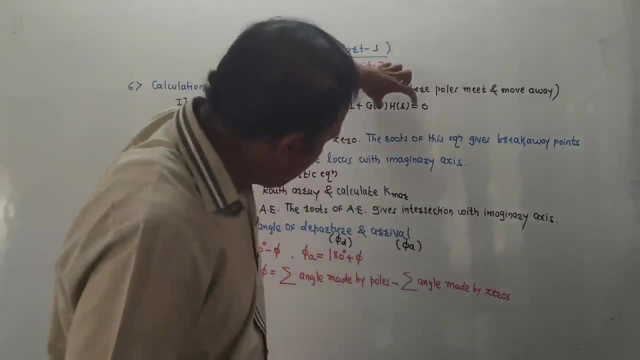 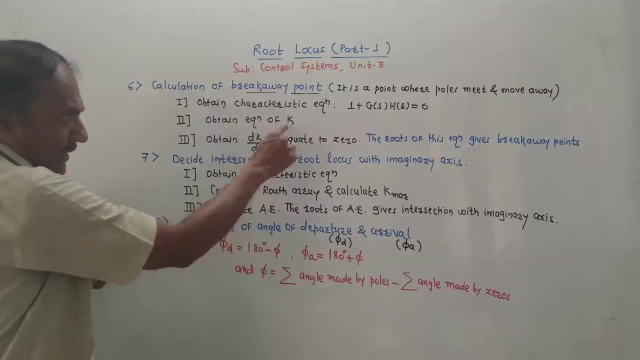 it. one plus G of s into H of s equals to zero. So by creating this equation we will get a characteristic equation. It will contain k term in it. So the second step is obtain equation of k, K from step 1. third step is take its derivative with respect to s, so obtain dk by ds and equate. 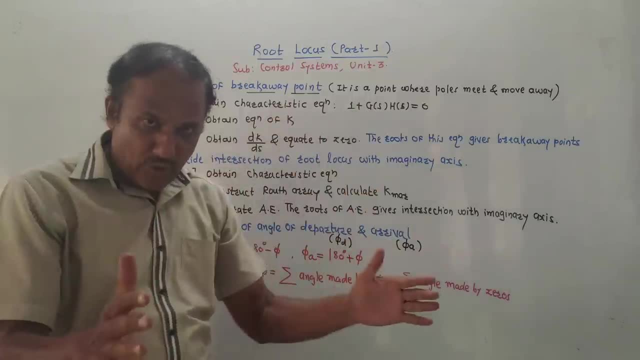 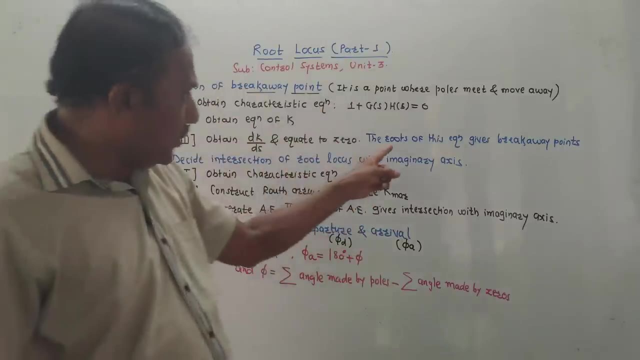 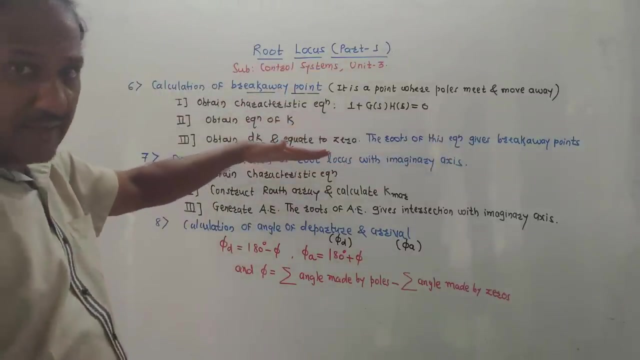 that to 0 means take its derivative dk by ds, equate it to 0 so you will get dk by ds is equal to 0. its roots to calculate the roots of this equation gives breakaway point. as i told you, we will solve numerical so this step will be more clear. see, if you want, take. 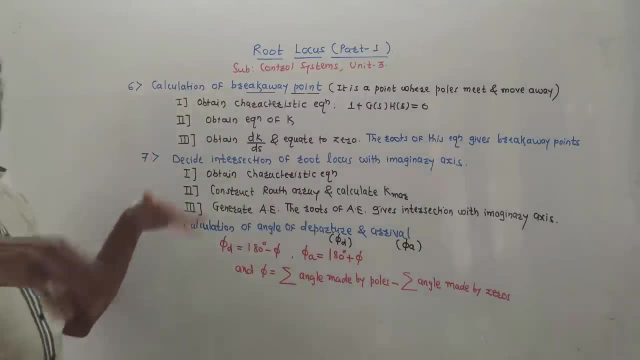 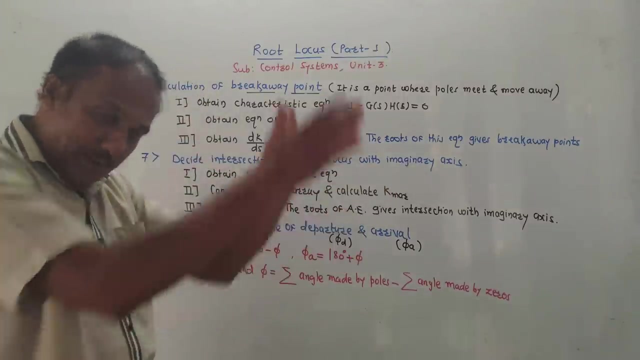 a screenshot. these rules are very important to solve numericals and if you get a theory question in question paper, then also you have to write these rules. next rule is: decide intersection of root locus with imaginary axis. how to calculate this means root locus to imaginary axis- imaginary. 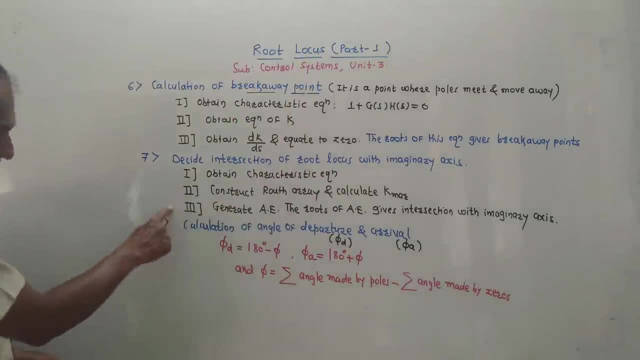 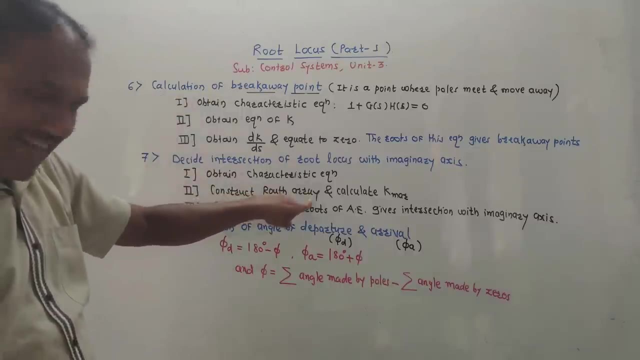 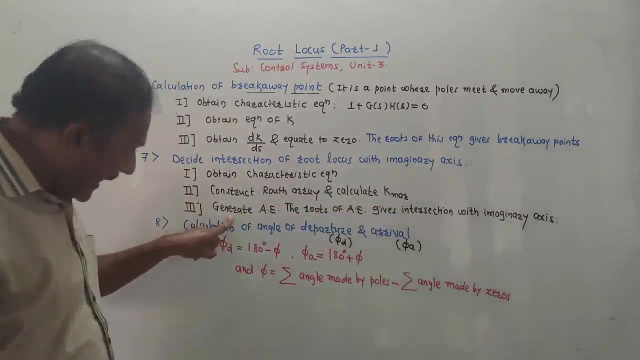 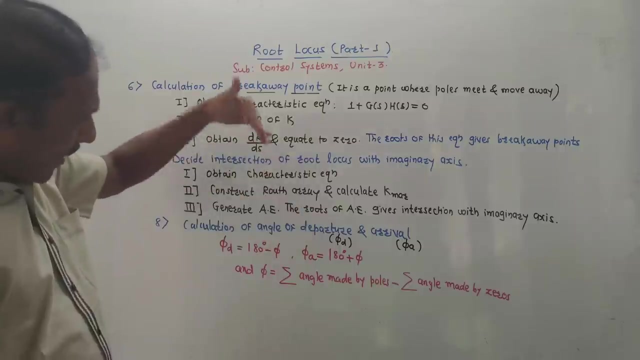 axis is y axis where it intersects. to calculate those points. these steps are: step one: obtain characteristic equation like this. second step: construct route array. route array to prepare and calculate k. marginal marginal value of k we need to calculate. third, calculate auxiliary equation. we have already learned. in case still, i will break up, brush up the things while solving. 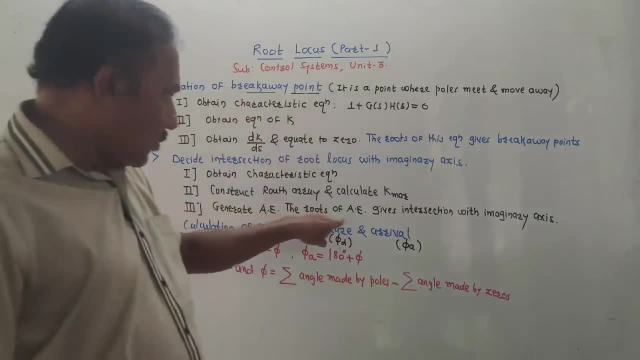 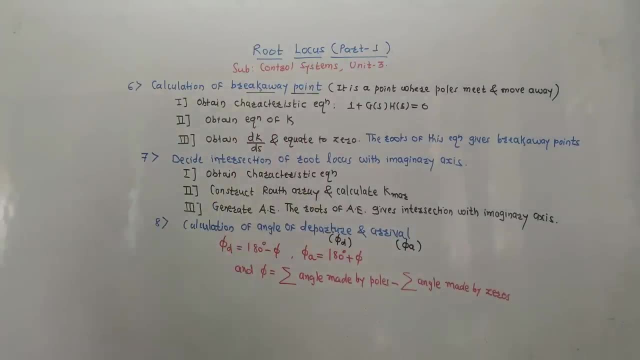 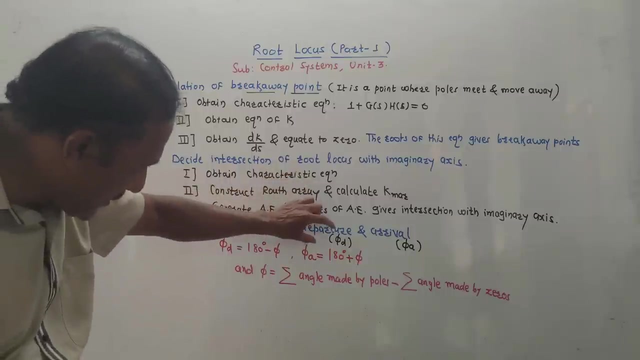 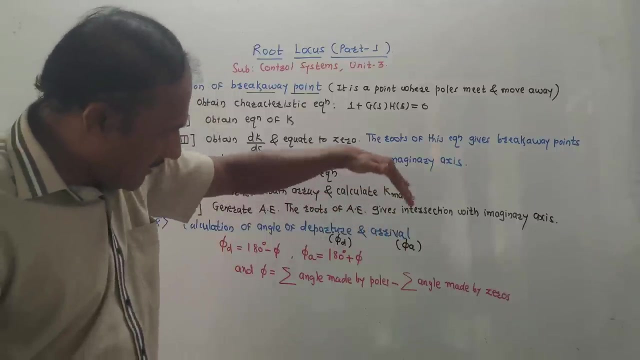 the numericals. so calculate auxiliary equation, then roots of auxiliary equation gives intersection with imaginary axis. last rule is calculation of angle of departure and arrival. year rule complex poles or complex zeros. angle of departure means from which angle is departing root locus, or angle of arrival, from which angle the branch is arriving. that is angle of arrival. it is phi d and phi a. 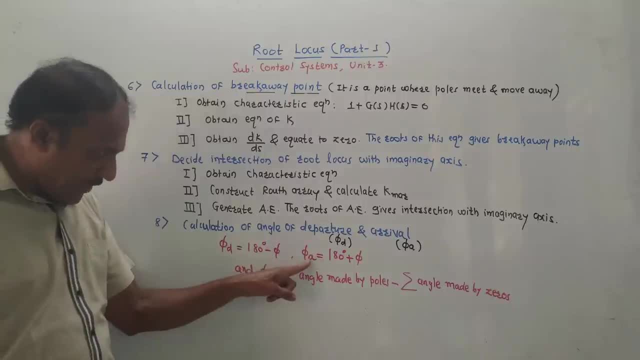 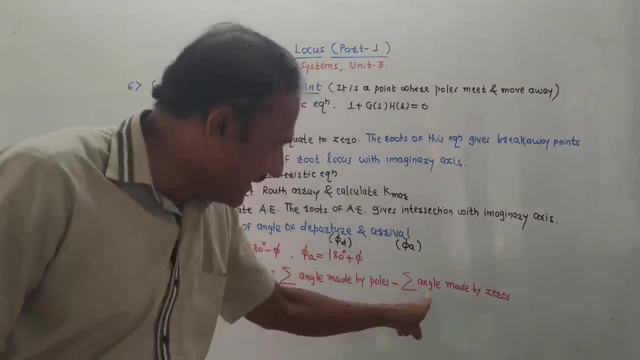 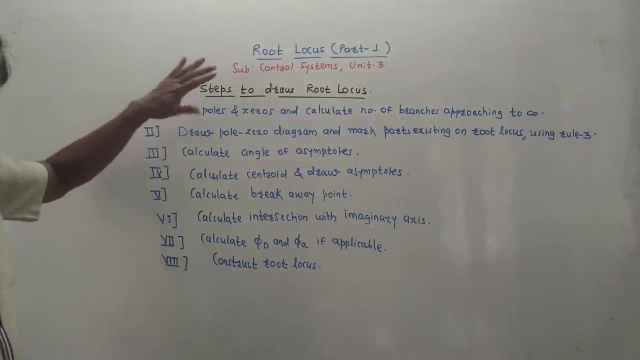 phi d formula is 180 degree minus phi. phi a angle of arrival is 180 degree plus phi, or phi's generalized formula is summation of angle made by poles minus summation of angle made by zeros. i have written the steps which are required to solve the numericals. that means to draw the root locus diagram. 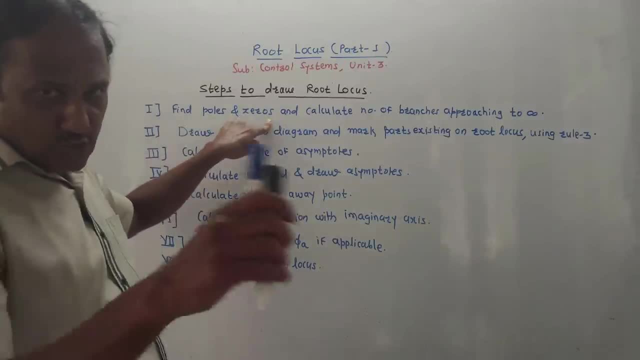 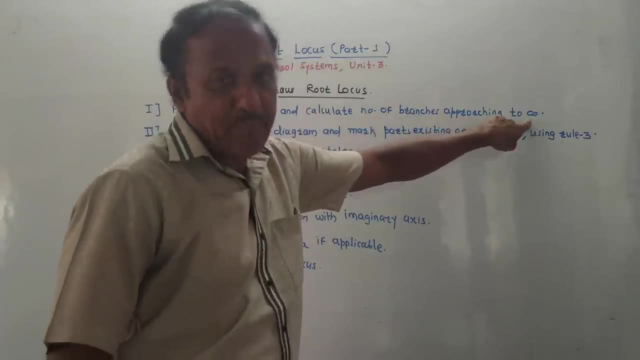 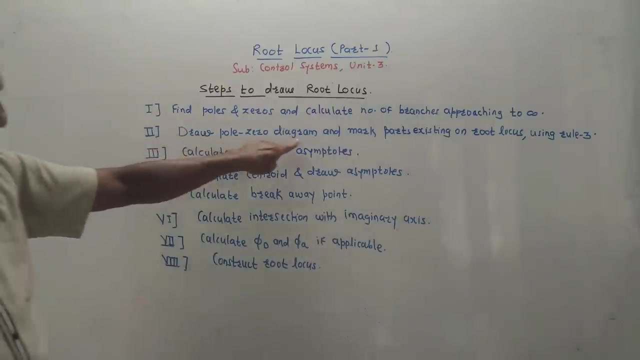 first step: find poles and zeros. as i have explained, zeros means roots of numerator, poles means roots of denominator and calculate number of branches approaching towards infinity. this rule we have studied. we will discuss it while solving the numericals. second step: draw pole zero diagram and mark parts existing on root locus using rule number three. third step: 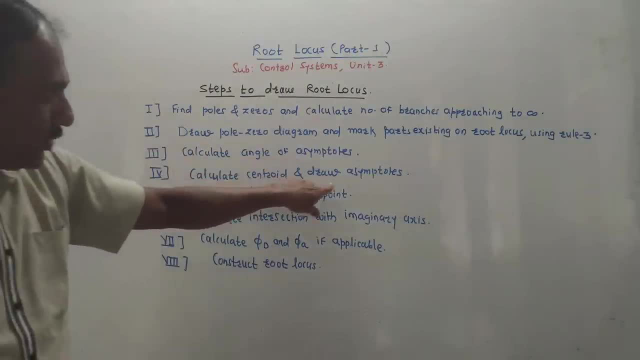 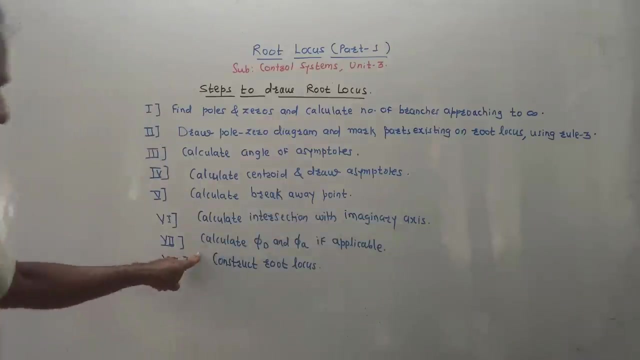 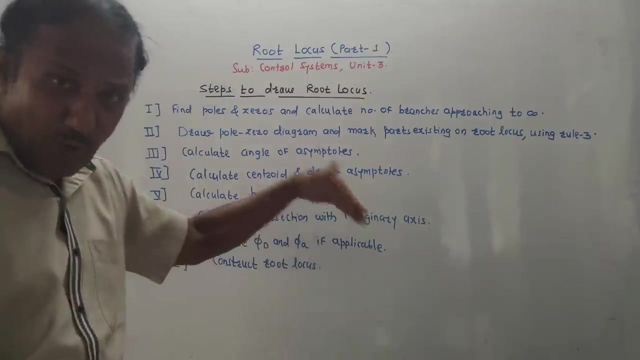 calculate angle of asymptotes. fourth, calculate centroid and draw asymptotes. asymptote centroid, which will travel towards infinity. next step, calculate breakaway point steps. already we have discussed the formula i have also told you. next, calculate intersection with imaginary axis. next, calculate phi. d means angle of departure and angle of arrival, if it is applicable, means in that problem. 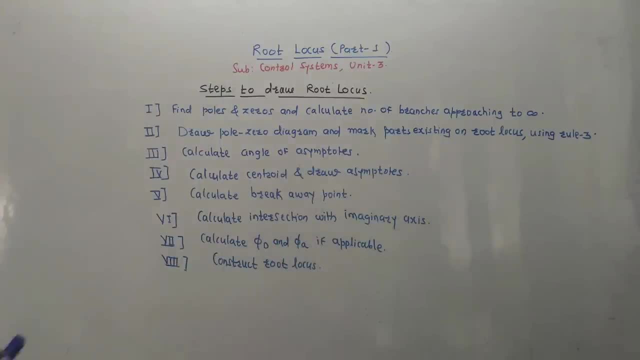 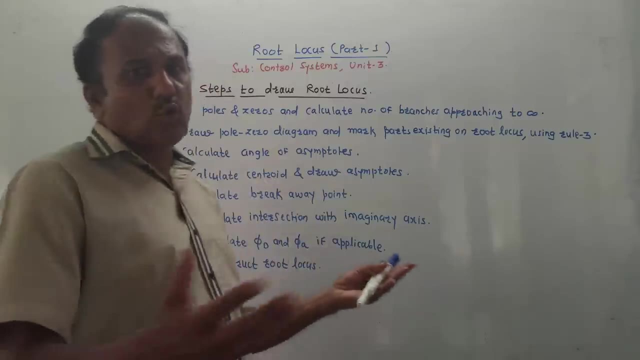 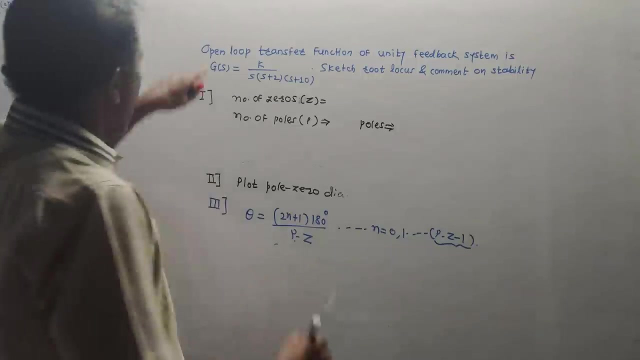 we have to do this calculation and last step is to construct the root locus and draw the root locus. construct the root locus. so let us make use of these rules and these steps to draw the root locus. so let us solve few numericals related to this. now let us solve one numerical. given numerical is open loop transfer function of unity feedback. 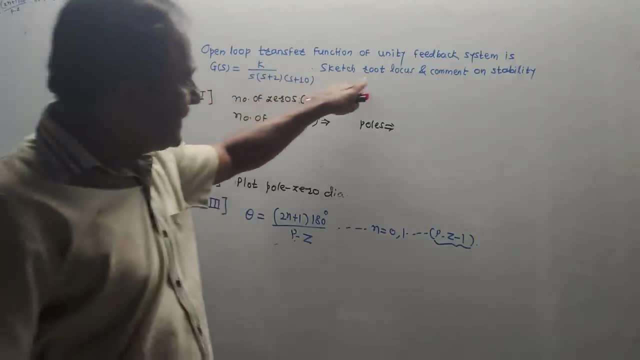 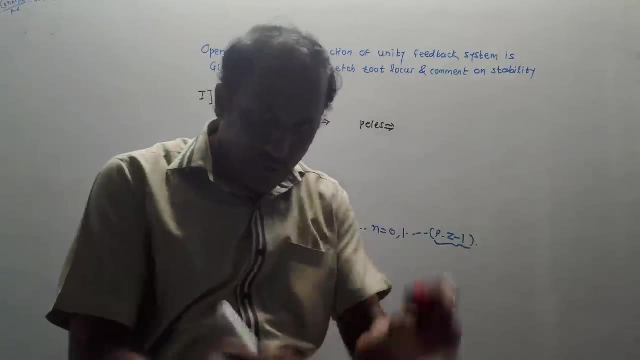 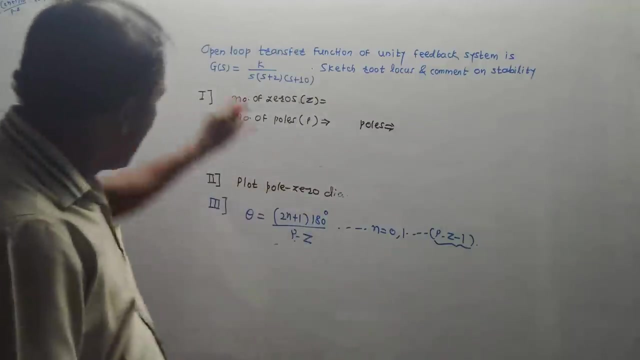 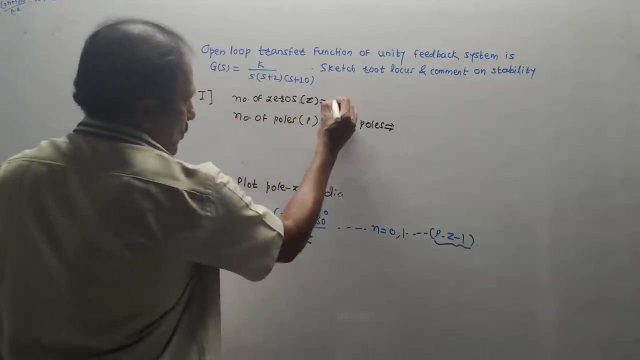 system is g of s. sketch the root locus and comment on the stability first part. they go make the thing simple. how to remember. the number of roots of the numerator is called zero. the number of roots of the denominator is called poles. look at given equation. in numerator there is constant k, there are no roots. so number of zeros z is equal to zero. 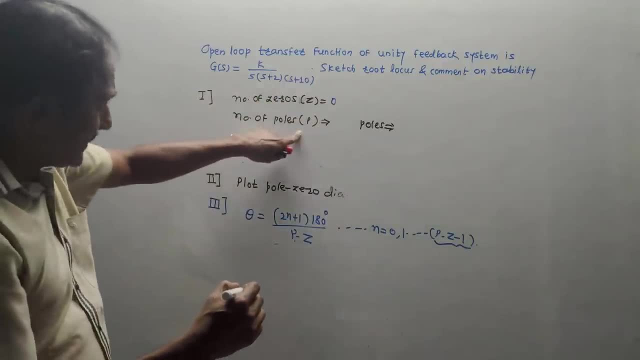 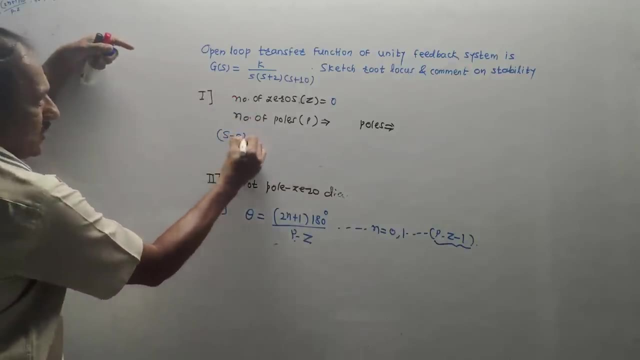 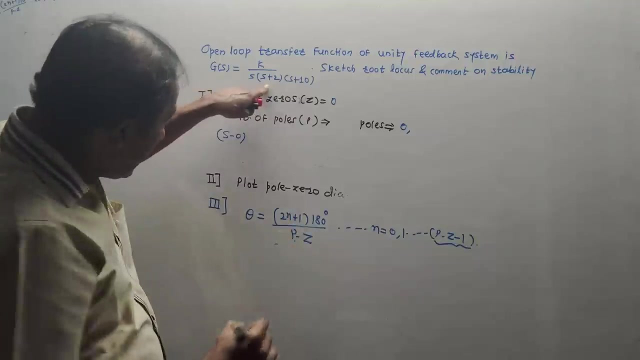 for simplicity i have written this from the beginning: number of poles. now see how many poles are there. see this first term, this is s. i can write this term as s minus zero. this is simple s. so i can write it as s minus zero. so first pole is at zero. second pole, this term is given as s plus two. remember the basic concept. 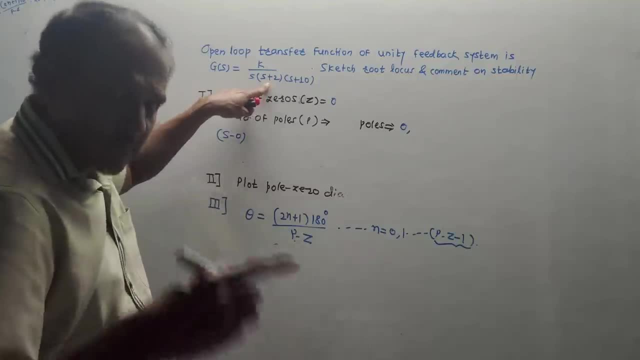 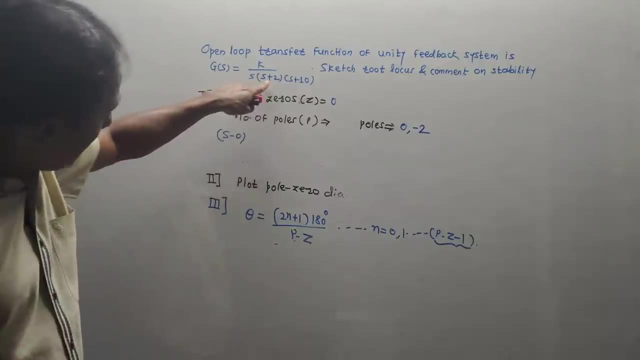 when we take out roots, ie pols. we are writing this. we are writing pols means roots, so we change this sign because s is plus two, so pole will be at minus two. very simple trick. if the sign was happening here, if it was minus, i would have written plus. 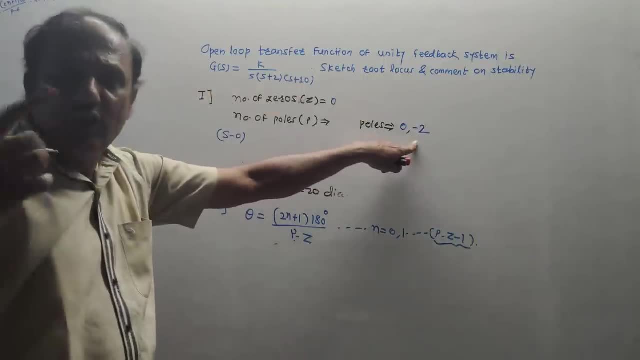 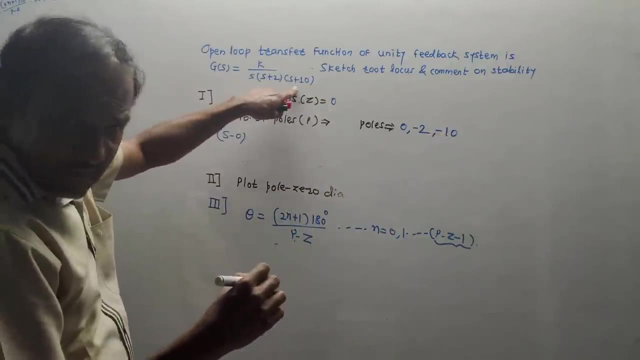 so it is plus. so if it was minus two, then this is the value at which the second pole is present: 3.. there is s plus ten pole will be at minus 10.. So there are three poles. one is at zero, another is at minus. 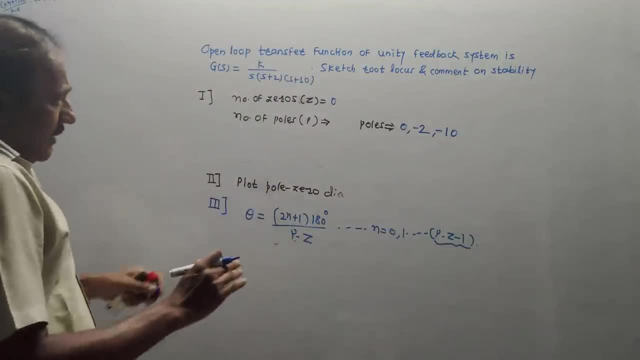 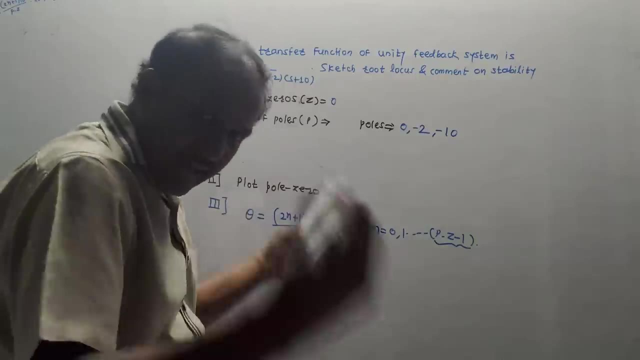 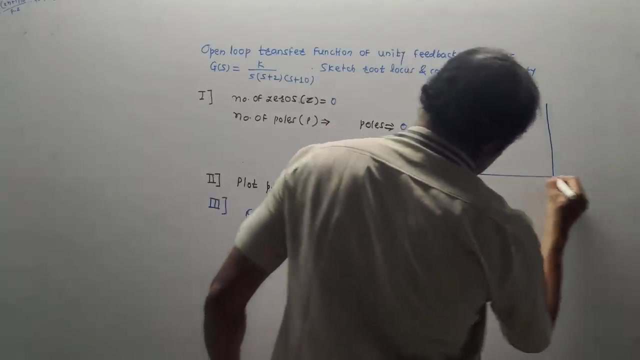 2, third is at minus 10.. Now in the second step, we have to plot the pole zero diagram and check which part is inside the root locus. How to do it? Drawing the pole zero diagram is a simple task. On this axis, write sigma, You can well write. on the x-axis, You can write: 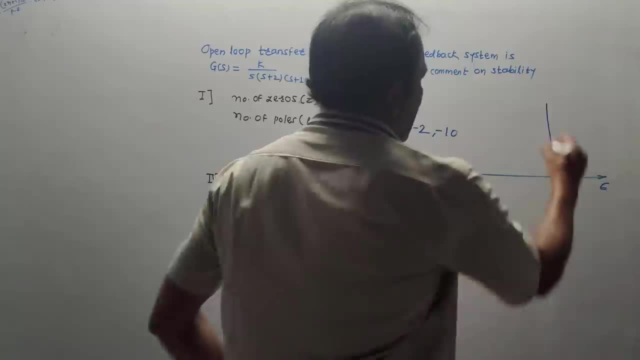 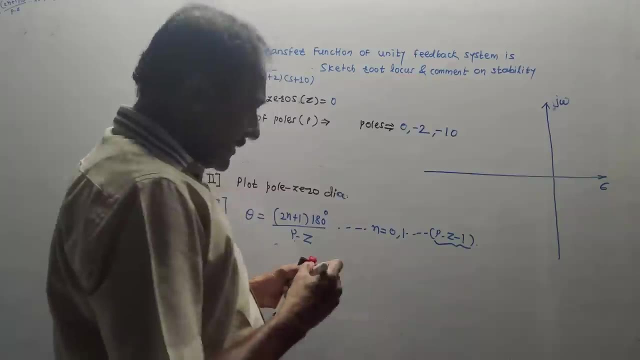 the real part as well. I am writing sigma. Sigma is the same as the real part. On the y-axis, write the imaginary part, or j, omega. Anything will do. Now see, let's mark the poles first. The first pole is at zero. Do remember the convention To mark zeros. we. 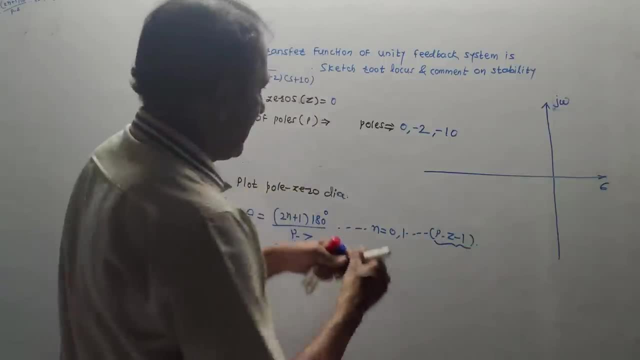 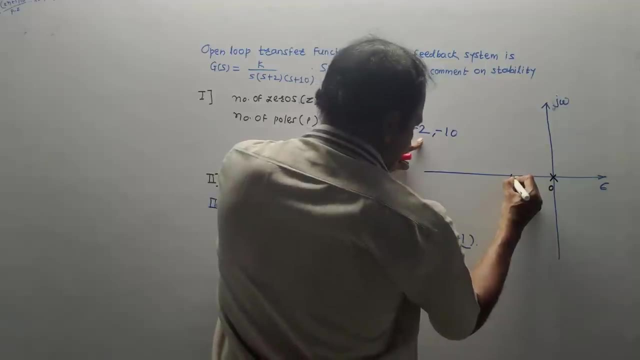 make a small circle To mark poles. we make a cross sign. So the first pole is at the origin. so I will mark this: This pole at origin. Second pole at minus 2.. Somewhere at minus 2.. Here let us say: 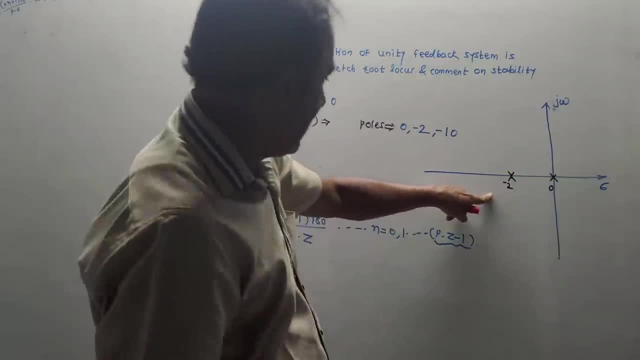 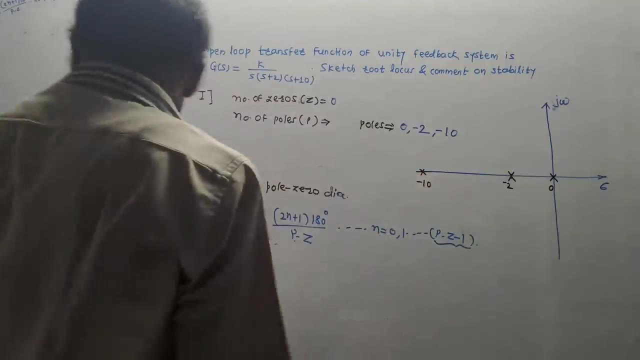 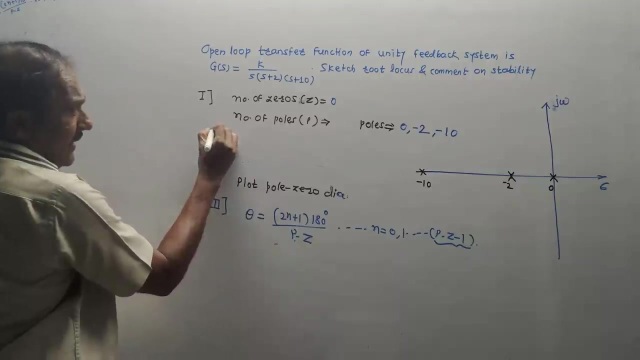 it is minus 2.. Remember, you have to make this on a graph paper to the scale. Third pole is at minus 10.. So suppose this is the value at minus 10.. I have made three poles like this: Okay, because there are three poles. Now, in this step we also have to calculate. 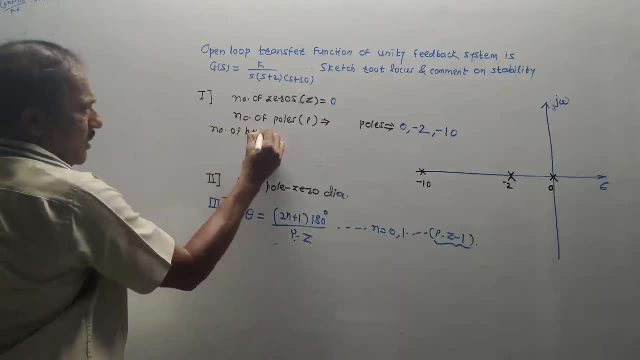 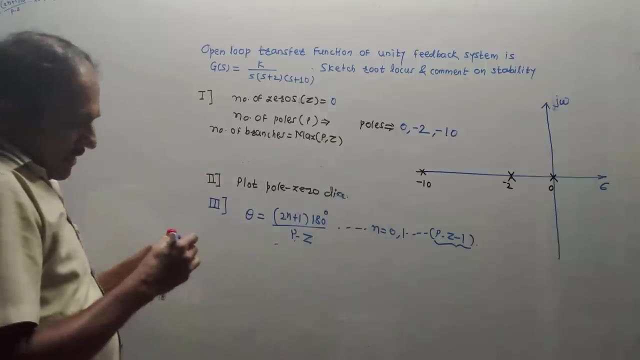 the number of branches. What is the number of branches? The number of branches is the number of branches. What formula have we already learnt? It is maximum of p, z. Now, p means the number of poles, z means the number of zeros, So in this formula it will be the. 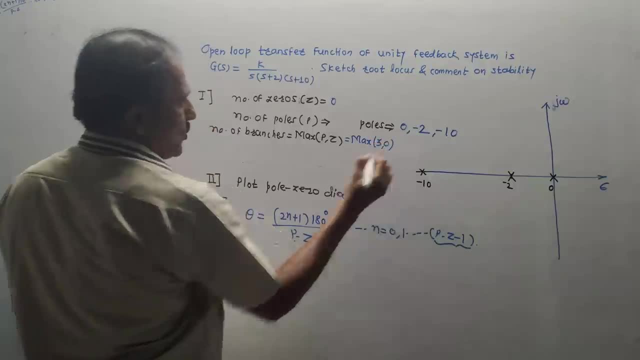 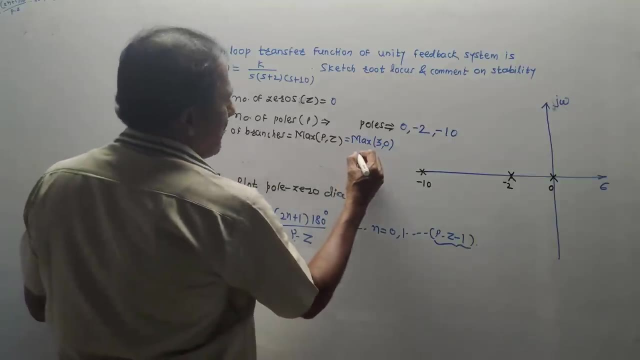 maximum of 3, 0. Because the number of poles are 3, the number of zeros are 0.. From this, what is the maximum value? 3.. So there will be three number of branches for the root locus. Along with that, we have to write the number of branches for the root locus as well. So 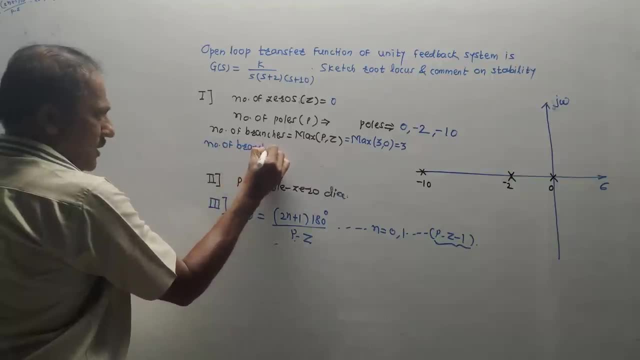 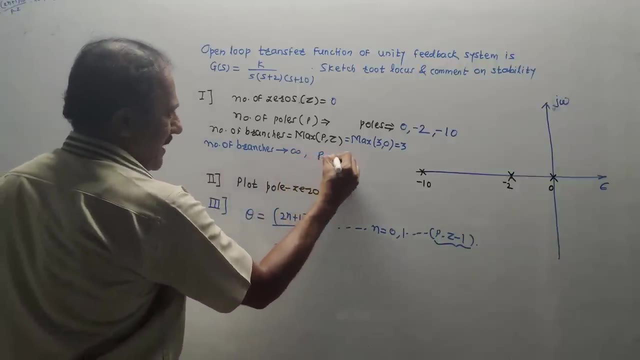 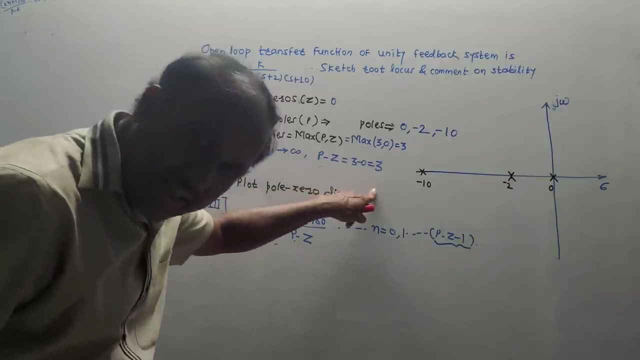 we have to write the number of branches tending towards infinity. I will mark the sign like this: tending towards infinity. What is the formula for this? It is p minus z, So it is 3 minus 0. It is equal to 3.. This means that three branches will tend towards infinity. 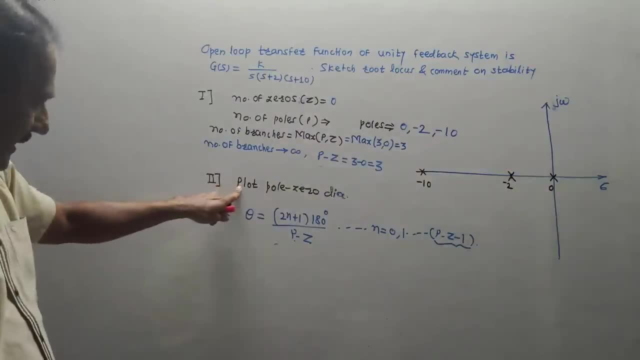 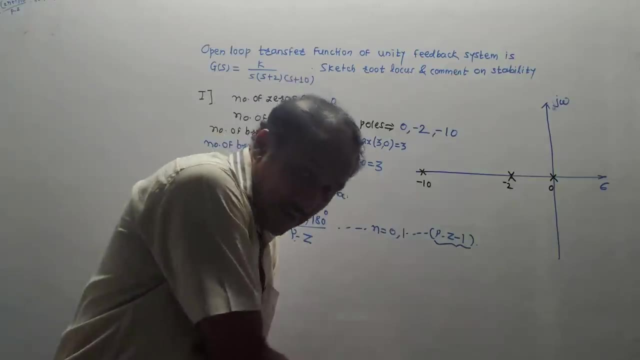 Now I have already marked the poles. So the second step I have done, that is, I have completed that is pole zero plot diagram. But in this diagram I have already written the number of branches. So in this diagram which portion is lying in the root locus that you need to? 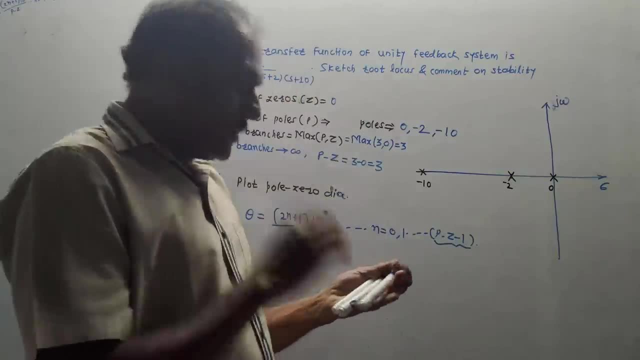 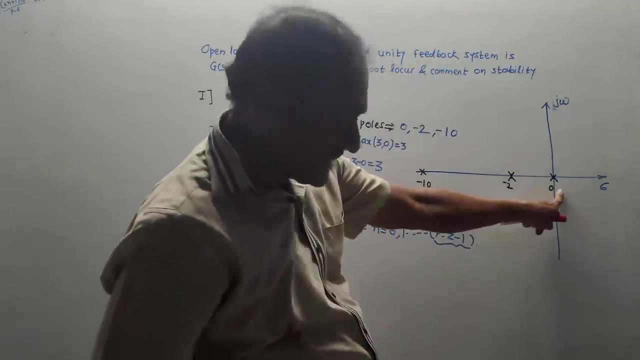 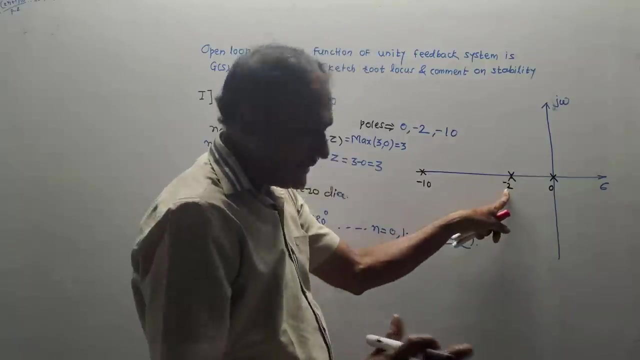 calculate Now. see, this is a very important step. Remember the rules. We have three poles. First pole: we have to move towards LHS, So we will start from here. After this, there is no pole. so don't think about pole at zero, Think about pole at minus 2.. How to predict? 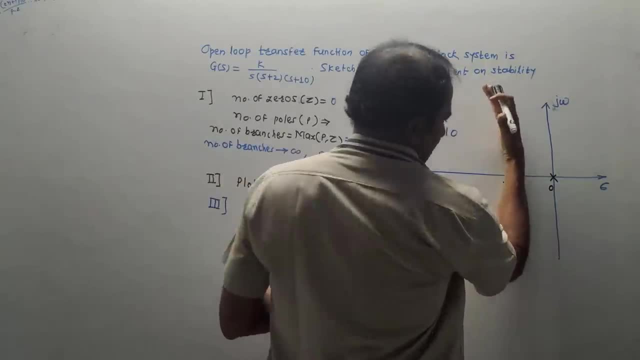 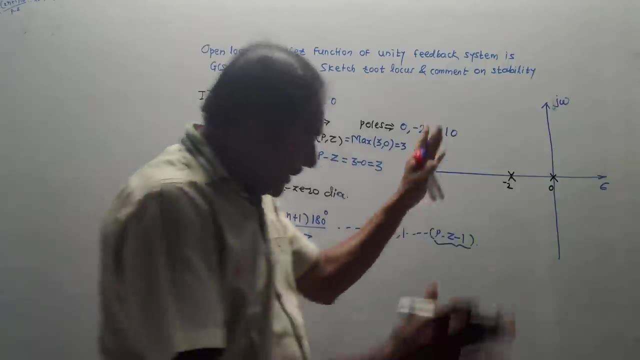 how to calculate From here, if I understand the vertical line like this, from here, the right hand side, how many poles and zeros are there? In this case, zero is not there. See, let's check. this time You don't have to differentiate between poles and zeros. 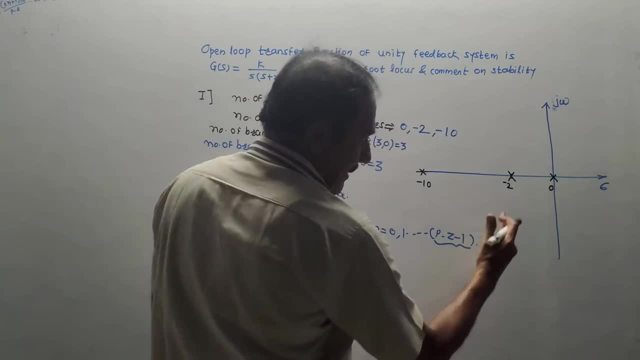 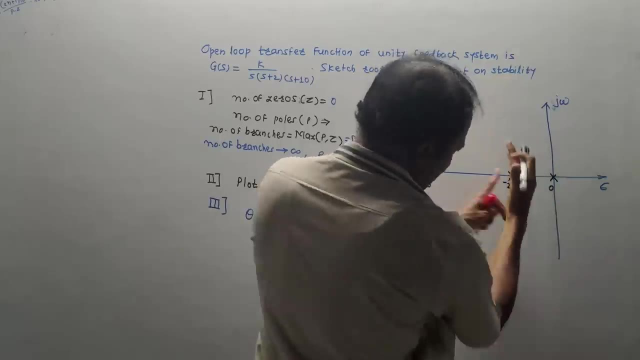 There are poles, there are zeros, there is a combination. Everything has to be calculated, Meaning I have skipped zero. This is the starting point. I have to move to the left If I draw a vertical line at minus 2, and think like this: related to minus 2,, how many? 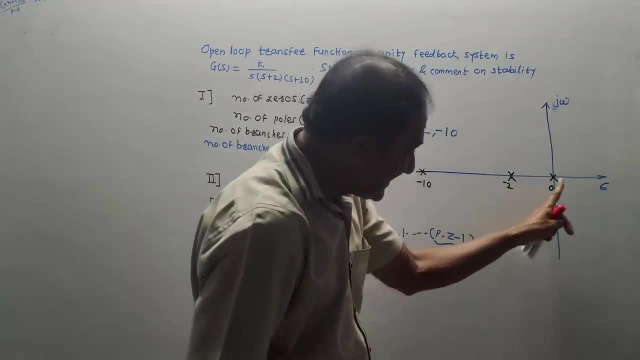 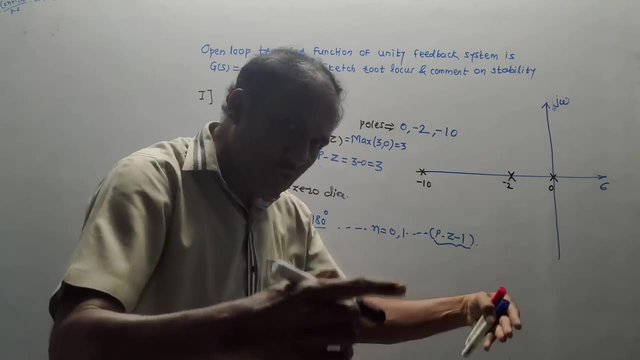 poles and zeros are there on the right hand side. There is only one pole on the right hand side. This number is one. One is odd number. It means that there is only one pole on the left hand side. If the number of poles and zeros is odd, then that portion is the part 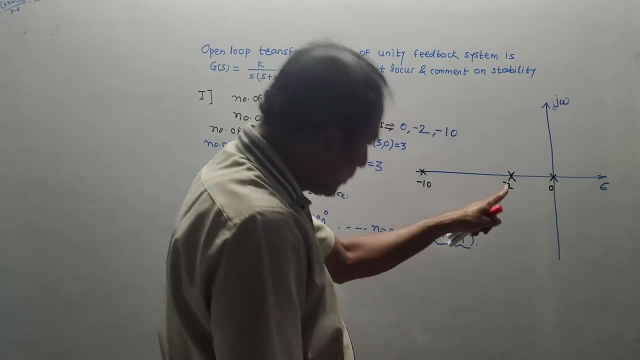 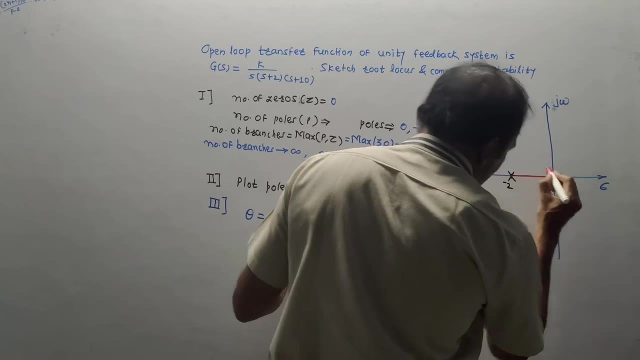 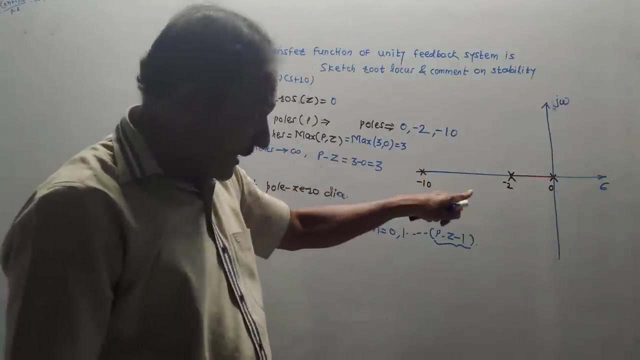 of root locus. So the conclusion will come that minus 2 to 0 is the part of root locus. The part of root locus has to be bold How to do in an exam. The diagram will be made from pencil, Just like how I have told you. it has to be made on graph paper on normal. 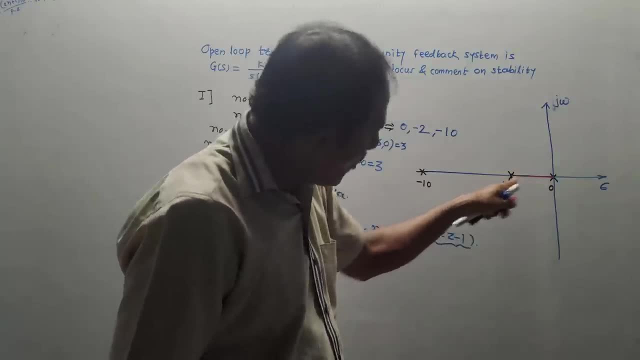 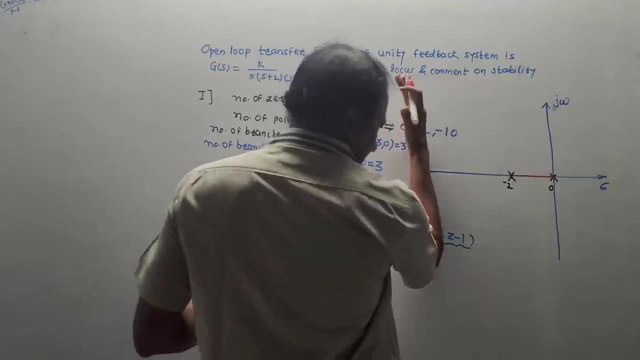 graph paper, The portion which is part of root locus. it has to be highlighted. That means you can draw it with a pencil. Now think like this: How to draw it From the left hand. We have to check on every pole related to minus 10.. 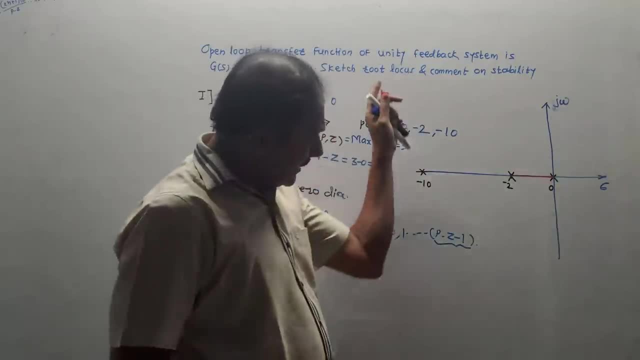 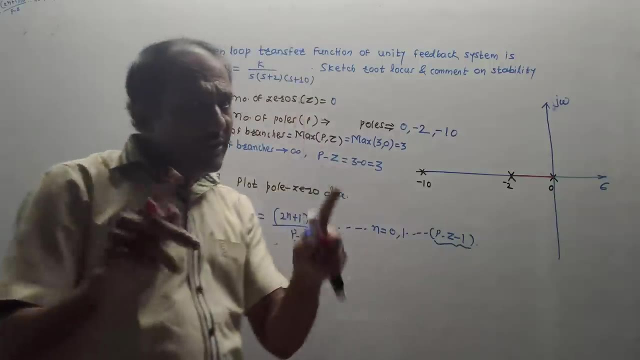 We will understand the vertical line like this On the right hand side: how many poles are there? Poles or zeros? anyone will work, But we don't have zeros in this numerical. So there are two number of poles. Two is even number. 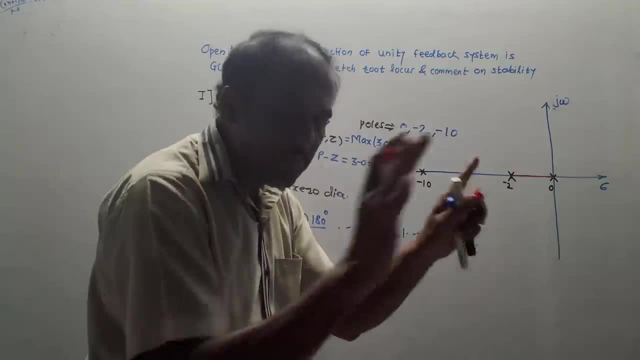 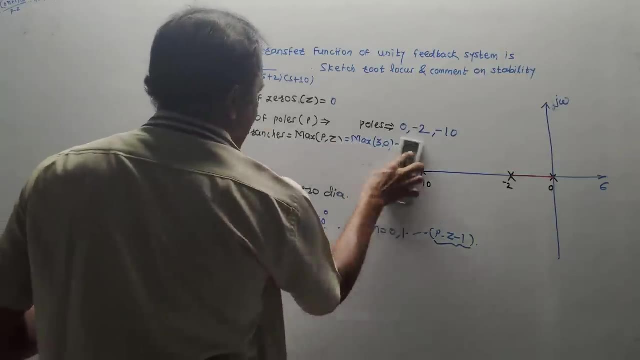 So minus 10 to minus 2 is not the part of root locus, The part which is not the part of root locus, we will keep it as it is Means, we will not highlight it, we will not make it bold Now. we have to calculate till infinity. 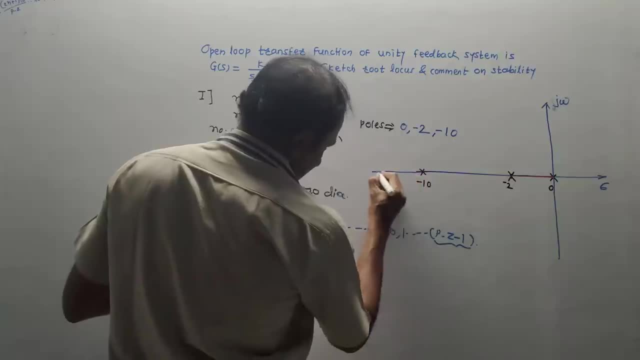 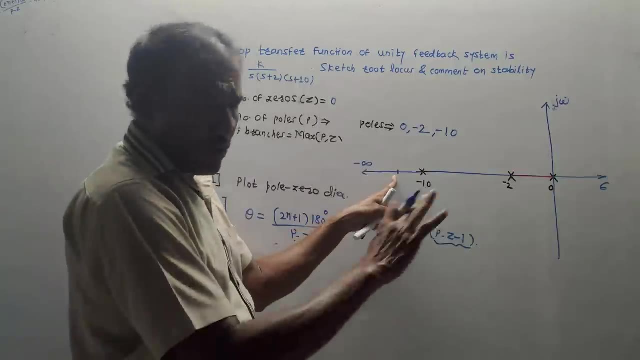 Means. I will extend the diagram and I will say this is minus infinity. Now see, take any point after minus 10.. Suppose this is the point. any point, I don't know what is the value of this point Here. we will think related to this. 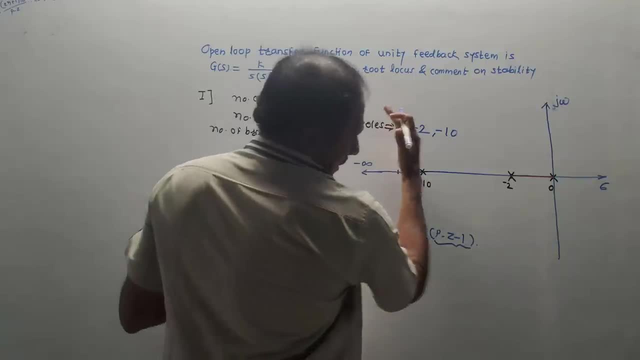 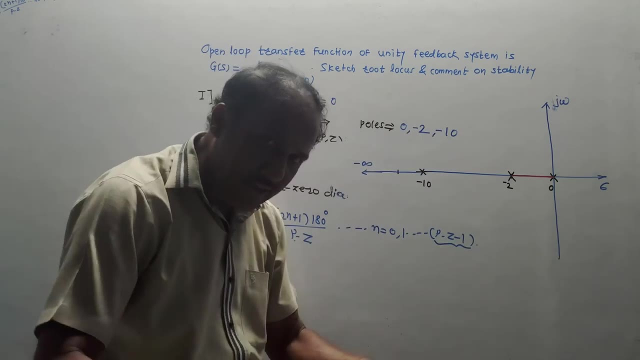 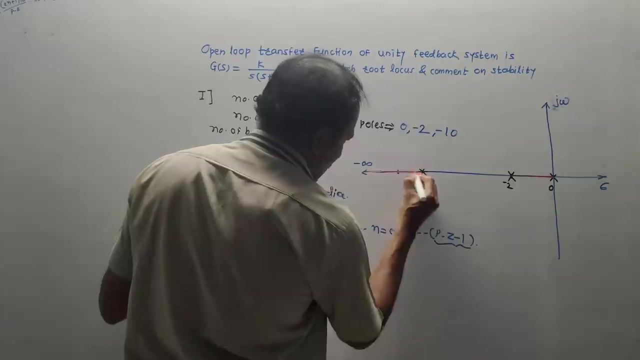 So, with respect to this point, at the RHS there are three number of poles. Three number of poles means number is 3, which is odd number. If there is odd number, then that is part of root locus. This means from minus infinity till 10, whatever portion is there, that is part of root locus. 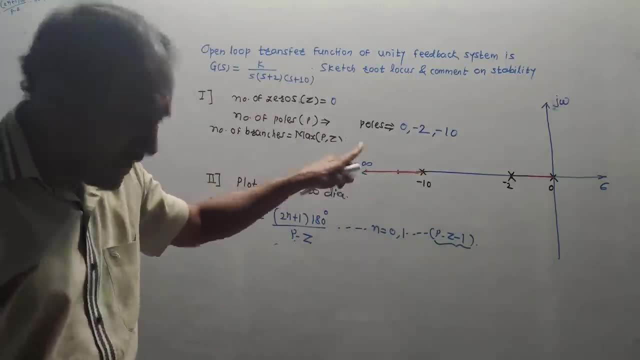 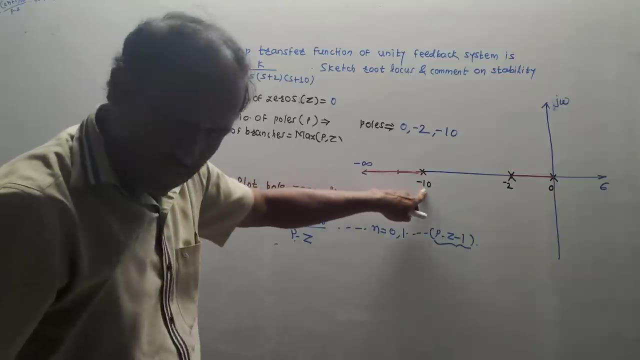 I have highlighted this. After this, if you take any value every time there will be three number of poles at the RHS And three is odd number. So every portion from minus infinity to minus 10 will be part of root locus. This is part of root locus. 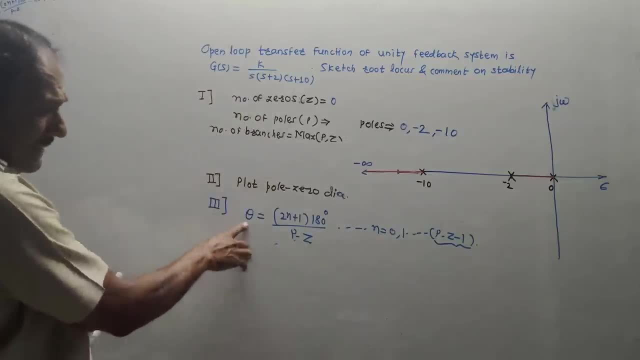 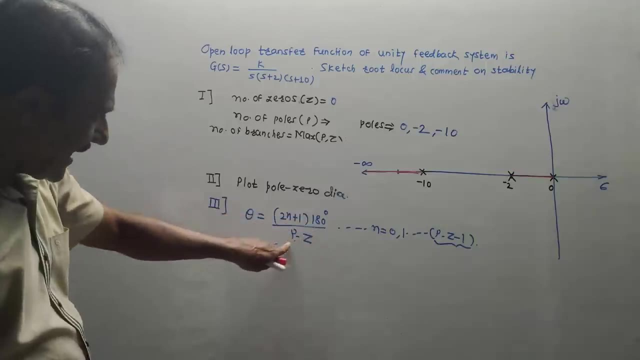 That is why I have highlighted it Now. third step: we have to calculate theta. Theta is angle of asymptotes. I have written a formula for that: 2n plus 1 into 180 degree upon p minus z. The range of n is 0, 1 up to p minus z minus 1.. 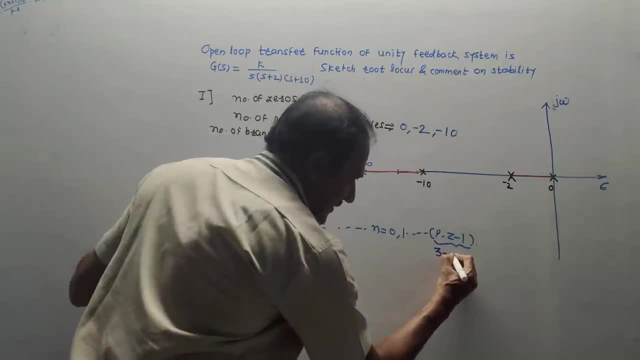 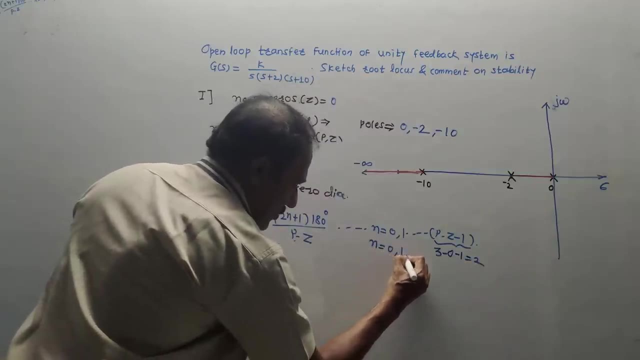 Means here: p means number of poles is 3.. z means number of 0, 0 is minus 1.. Its answer is 2. Means values of n will be 0,, 1, 2 in this numerical. 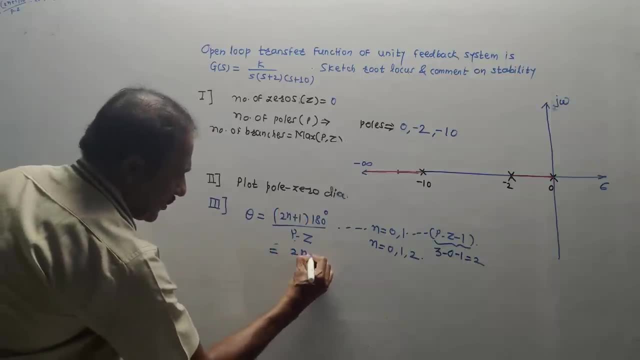 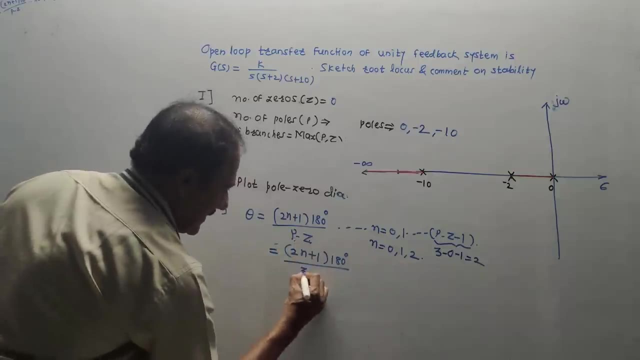 Now let us first simplify this equation. I will write it like this: 2n plus 1 into 180 degree upon p minus 1. Means 3 minus 0. This will be just 3.. So I am writing it like this: 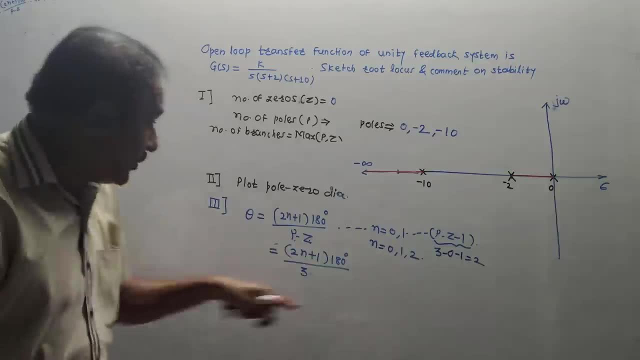 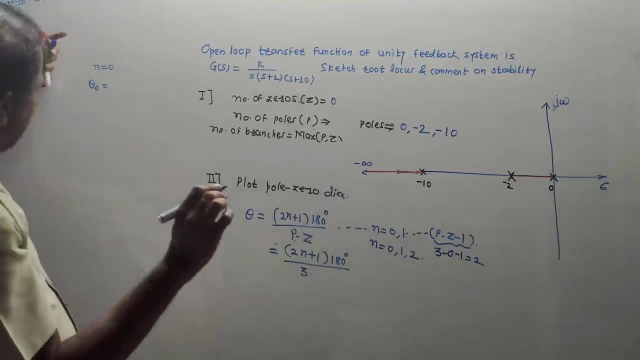 3 minus 0, that is 3.. Now we have to put different values of n. So first value n is equal to 0. For this theta is 0. Any notation will work. So this value is theta 0, because I am putting n is equal to 0. 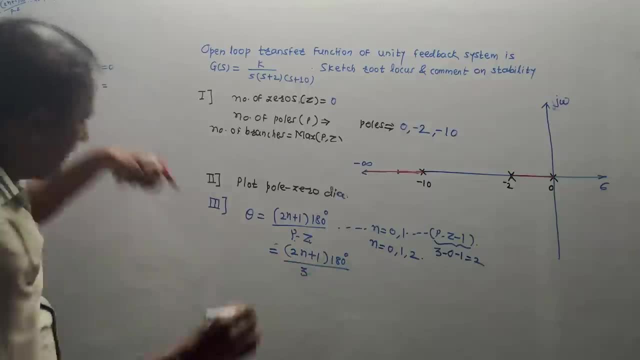 Wherever n is 0 has to be put 0 into 2 is 0. So it becomes 1 into 180 degree upon 3.. So theta 0's answer is 60 degree, Theta 1.. Theta 1.. 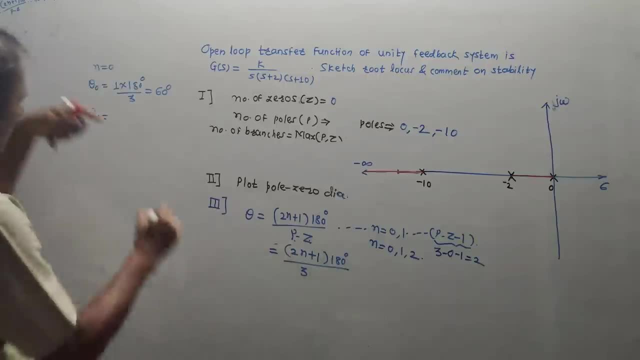 Means we have to put n's value 1.. So 1 into 2 is 2.. So this will be 2 plus 1 into 180 degree upon 3.. So its answer is 180 degree. This is 2 plus 1 into 3.. 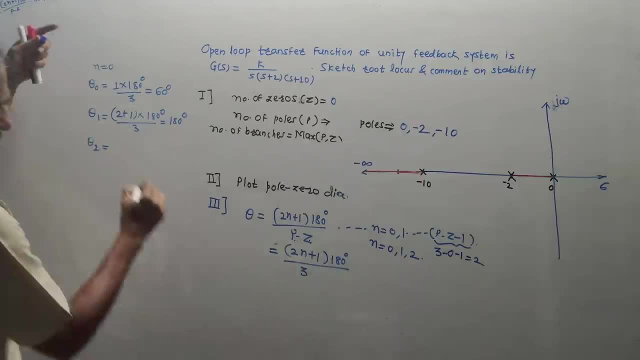 Theta 2. Means we have to put n's value 2.. So this will be: 2 into 2 is 4 plus 1 into 180 degree upon 3.. So if you calculate this answer, this will be 300 degree. 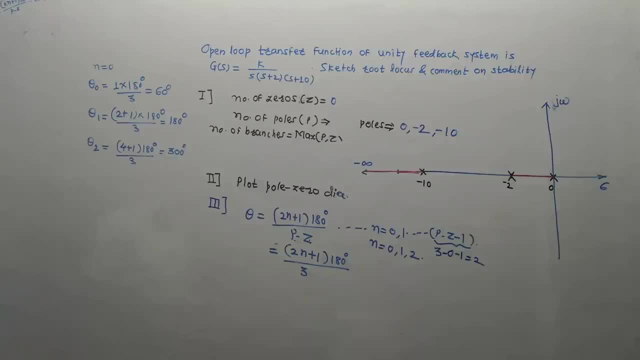 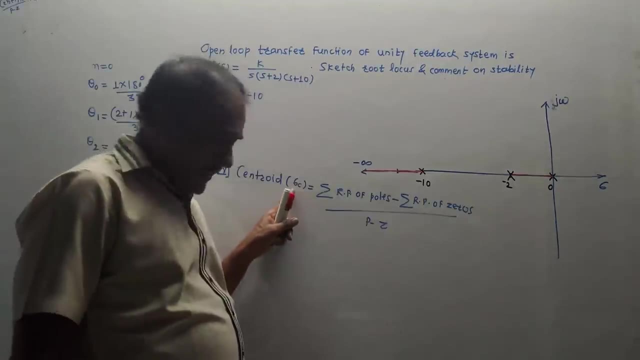 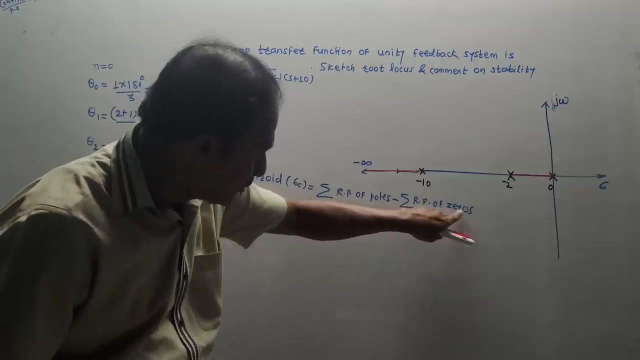 This means angle of asymptotes are 60 degree, 180 degree and 300 degree respective. Next tip: we have to calculate centroid. Formula of centroid is summation of real part of poles. Rb means real part, Real part of poles minus summation of real parts of zeros upon p minus z. 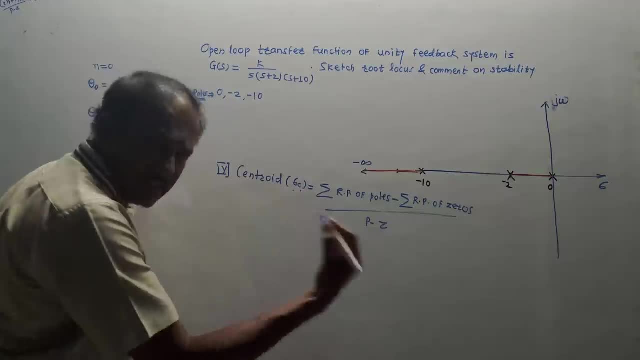 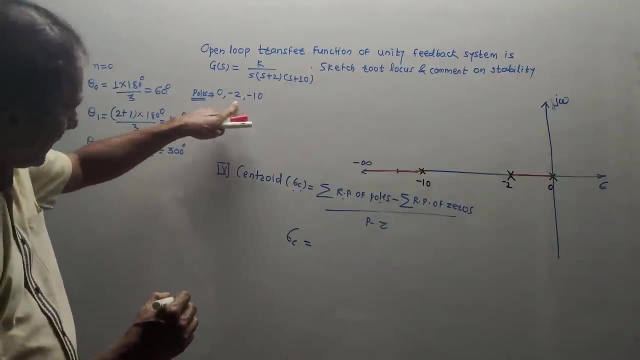 So let us put the values Notation sigma c or sigma, any notation will work. So sigma c is equals to summation of real parts of poles. Poles are 0, minus 2, minus 10.. Do remember: this is real part. 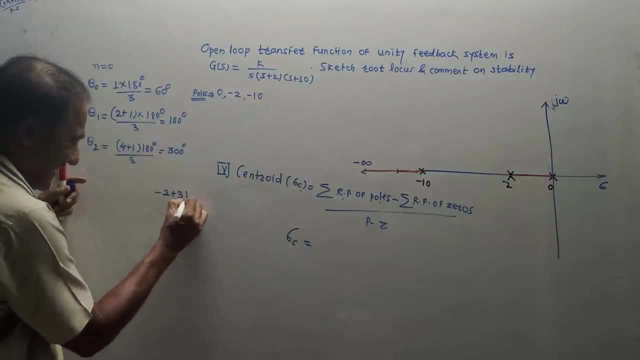 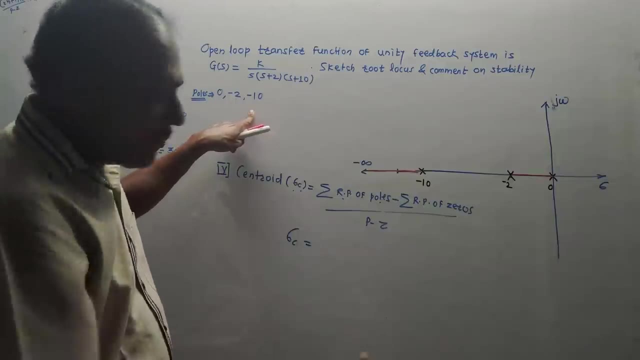 Means if pole is like this: Minus 2 plus 3 is 6.. So real part means only we take minus 2.. Likewise, So given values are already real. These are not complex terms, So I will put the values. 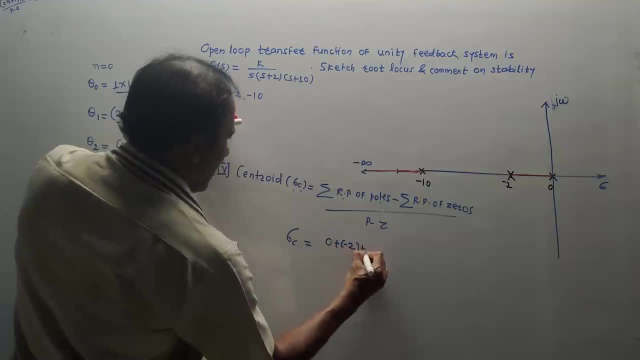 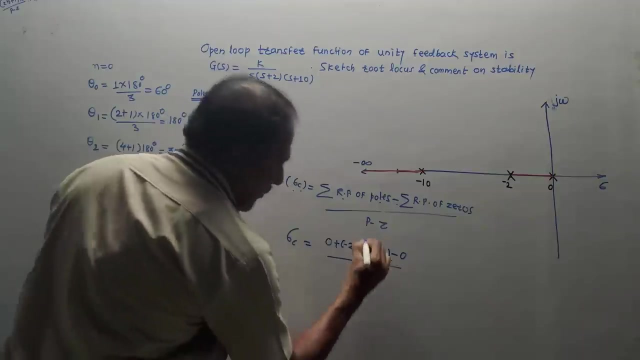 0 plus minus 2 plus minus 10.. Already the values are real. We have to put with sign Minus summation of real parts of zeros. There are no zeros in this, So this term is absent, So I will write minus 0 upon p, minus z. 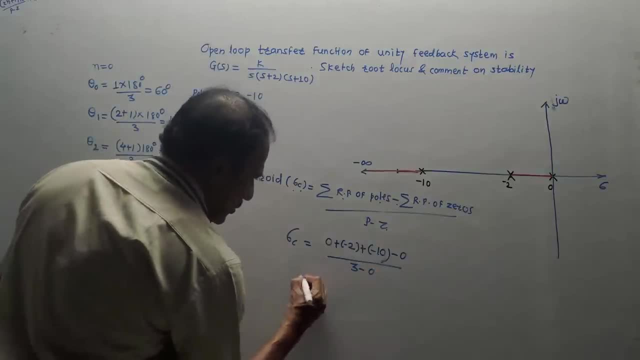 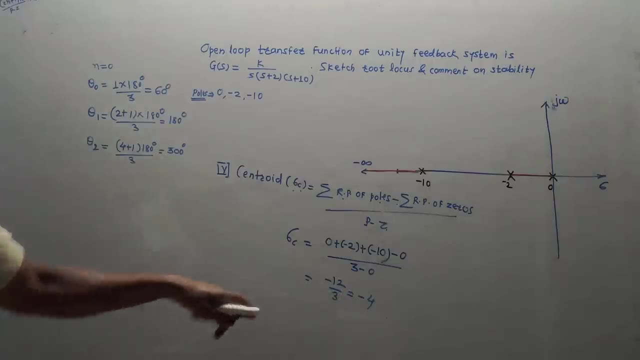 p means number of poles, z means number of zeros, So it is 3 minus 0.. So this answer will be this is minus 12 upon 3 is equals to minus 4.. This means centroid we got it is at minus 4.. 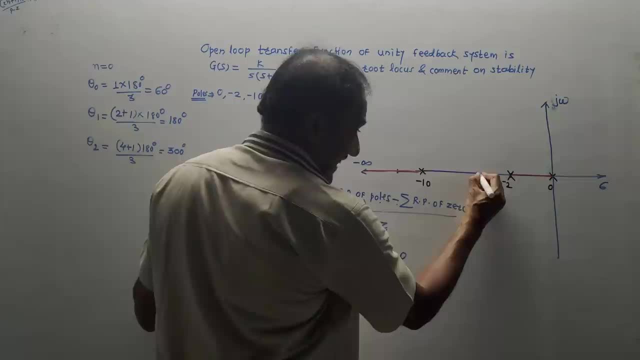 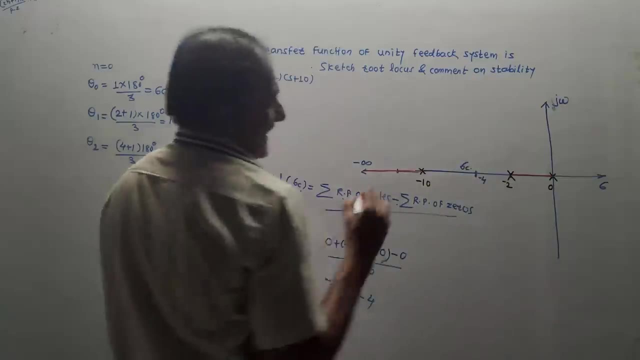 So let us mark this value. As I told you, you have to draw it to the scale. Let us say: this is minus 4.. This value is minus 4.. And this is sigma c. Now, what is the important part? 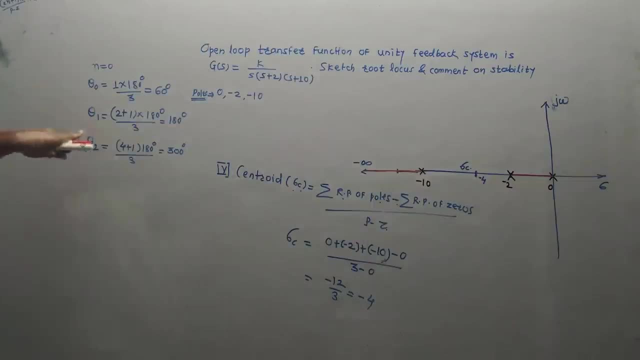 We will calculate centroid once. So we have calculated theta 0,, theta 1, theta 2.. We have to mark this. These are called asymptotes. We have to mark with dotted lines How to mark it. First angle is 60 degree. 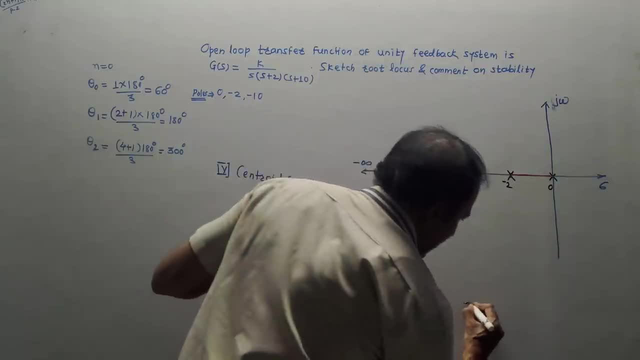 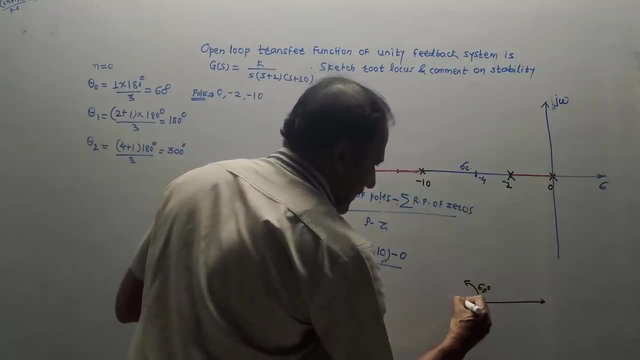 So from this point see, We have to measure angle. if this is x axis, So we have to measure angle like this, So we need to measure it 60 degree. So this 60 degree means like somewhere like this. It will be like this: 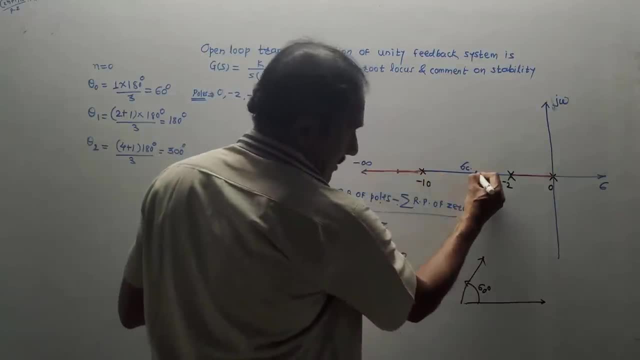 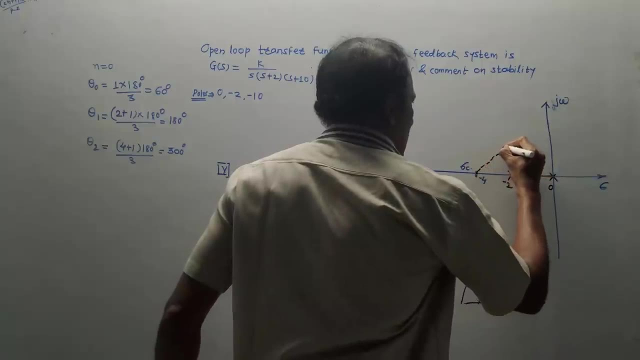 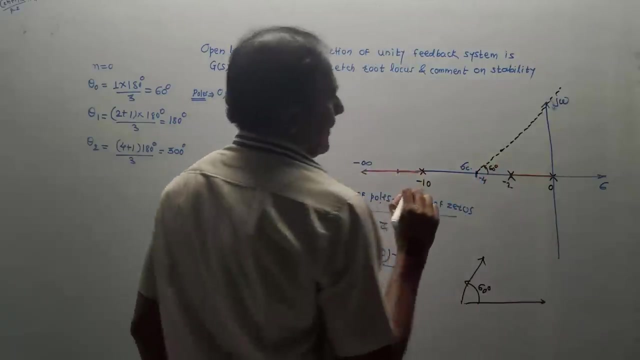 Likewise. from this point we have to draw asymptotes. Angle is 60 degree plus 60 degree. First value is 60 degree. Draw a dotted line corresponding to 60 degree. This angle is 60 degree. Second, centroid is at 180 degree. 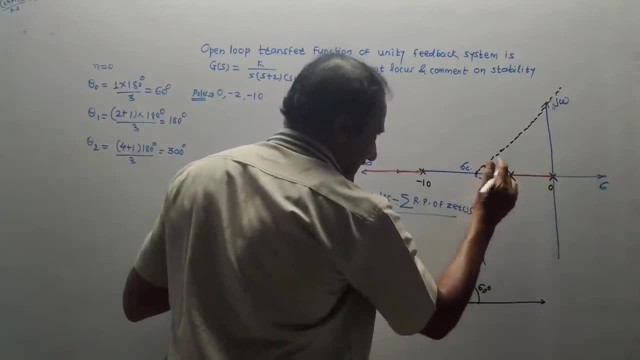 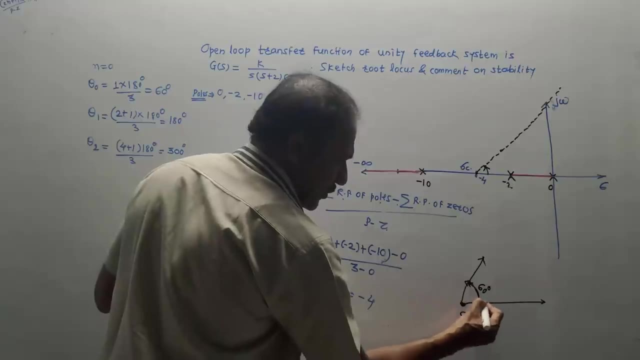 Same way. see Here when I have calculated: 60 degree angle is like: this Means we are measuring like this Same way: if you measure 180 degree- Suppose this is original- 180 degree will be like this: 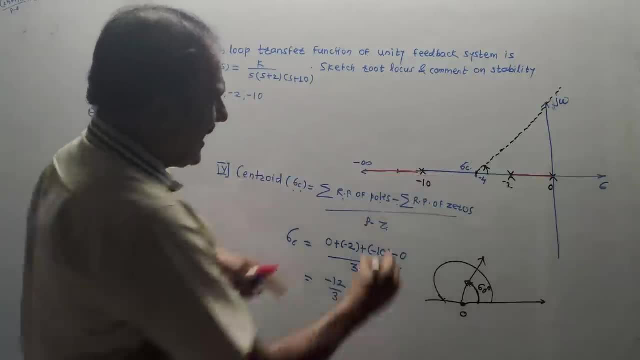 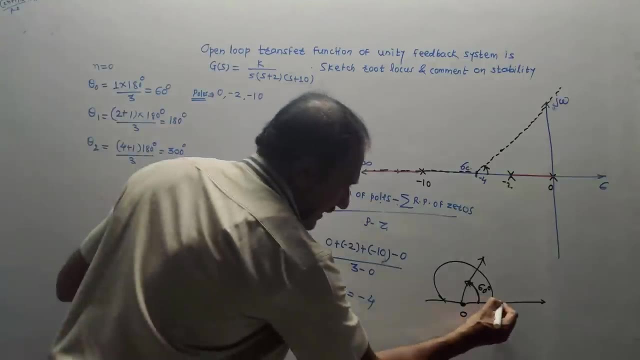 It will come till here. So I have already drawn a line, So a dotted line will come on this Like this. Third, it is at 300 degree. Same technique from here Means with respect to real axis. 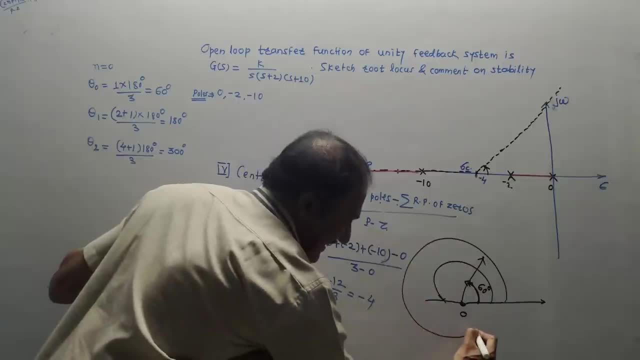 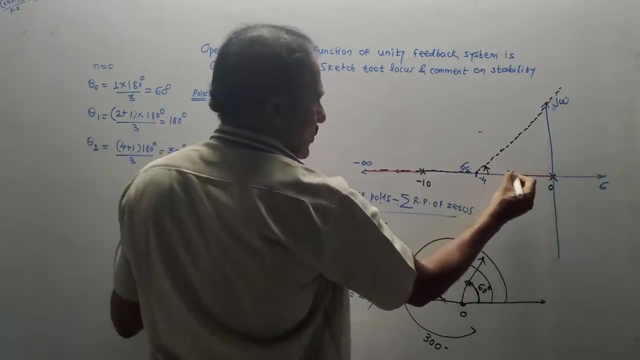 This is original With respect to real axis. we have to measure like this. We have to measure 300 degree till here. So we will measure like this. So this angle, 300 degree, will be somewhere here. I will mark it here. 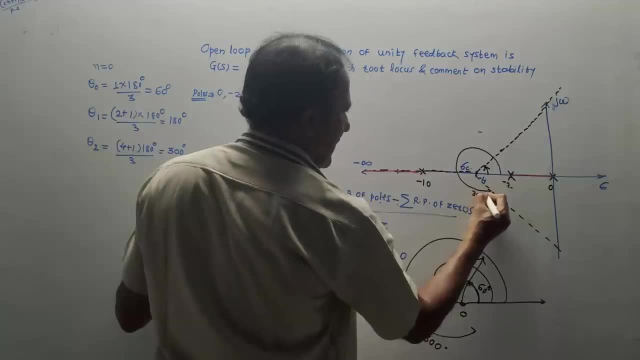 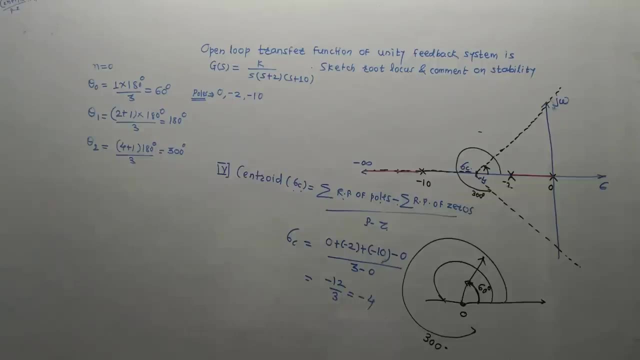 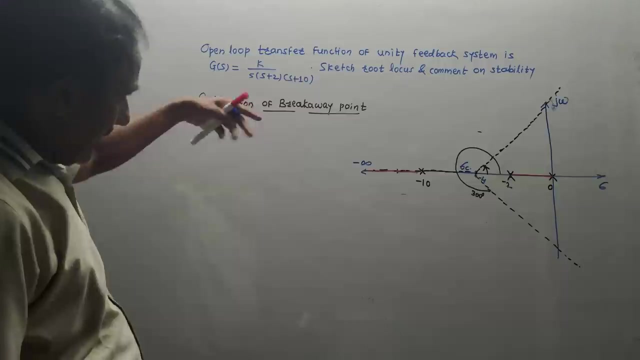 This angle will be 300 degree, Like this. So this is the way how to mark the asymptotes, If you have the values of angles. Next step: calculation of break-away point. We have written this in rules. What is the requirement? 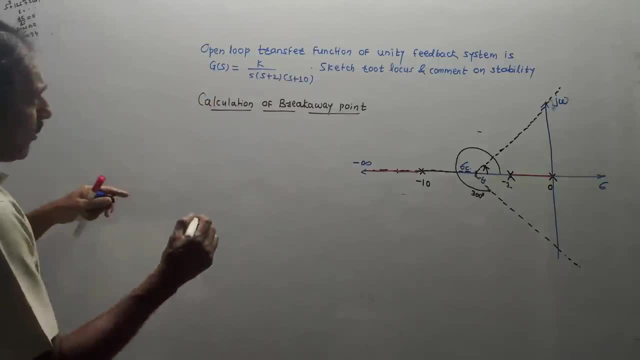 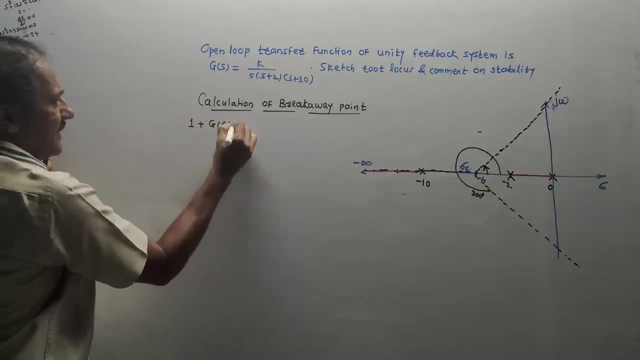 Presently we are talking about this particular numerical. Now see. First step is we need to generate the characteristic equation. How to do it? 1 plus g of s into h of s is equal to 0.. In unity feedback system, h of s is 1.. 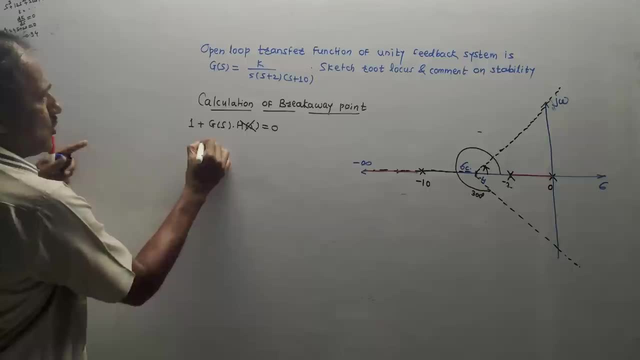 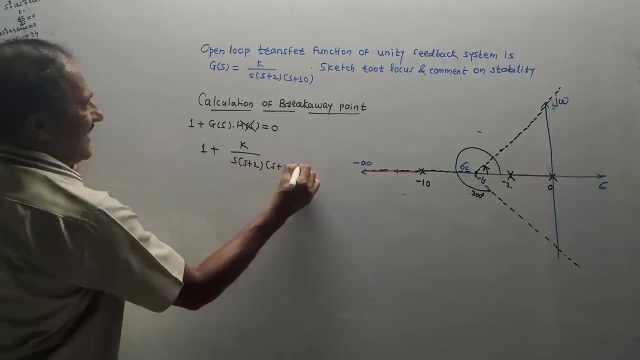 So h of s will be cut from here. Put the value of g of s, which is given in the equation- It is k upon s- into s plus 2. s plus 10 is equal to 0.. Take LCM: We have to multiply everything with 1.. 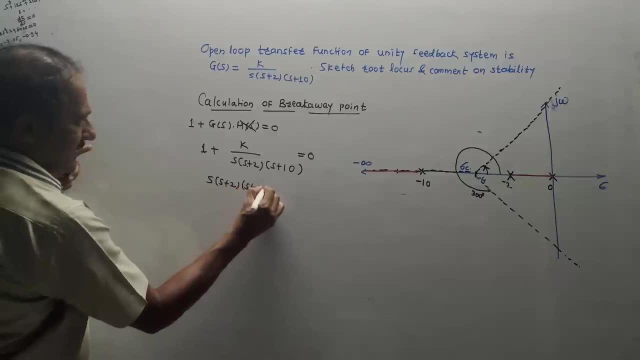 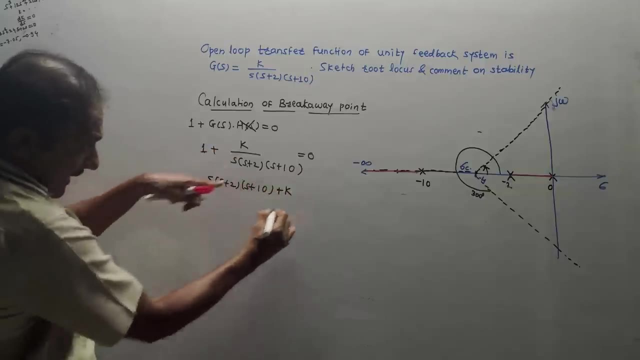 So it becomes s into s plus 2, s plus 10.. This is 1 into a Plus k. remains as it is, Divided by this whole term will come. But in RHS it is 0. Divided by this whole term will come. 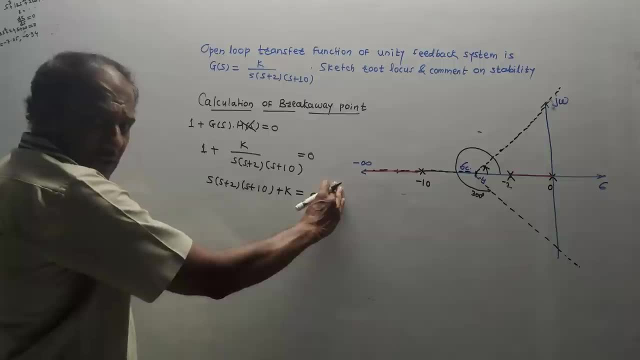 In RHS it is 0. So if I transfer this term to denominator here, it will also become 0. So I am not writing it, I am skipping it. Take LCM, Multiply this whole term with 1.. 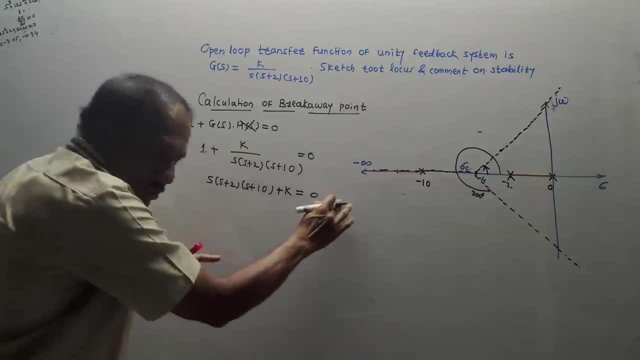 Write plus k Divided by this, whole term will come, But in RHS it is 0. So if I transfer this term to denominator here, it will also become 0. So I am skipping it. Let us expand this summation. 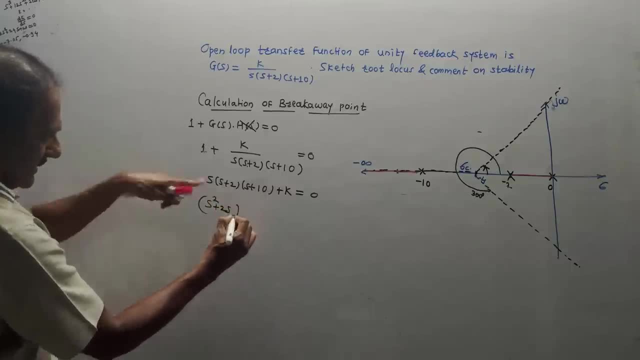 I am writing it like this: S square plus 2, s. I mean multiply it with s In second bracket. s plus 10 plus k is equal to 0.. Let us simplify further: S cube, We will multiply it with s square. 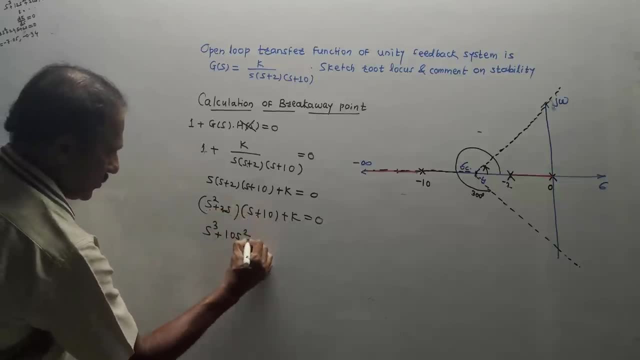 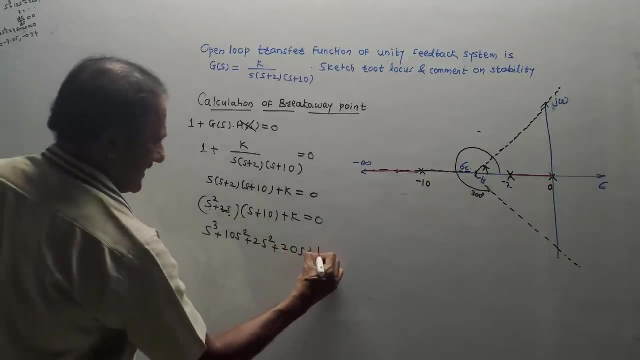 S cube plus s square into 10.. 10 s square plus 2 s into s, plus 2 s square plus 2 s into 10.. It is 20 s plus k is equal to 0.. So we have got the equation. 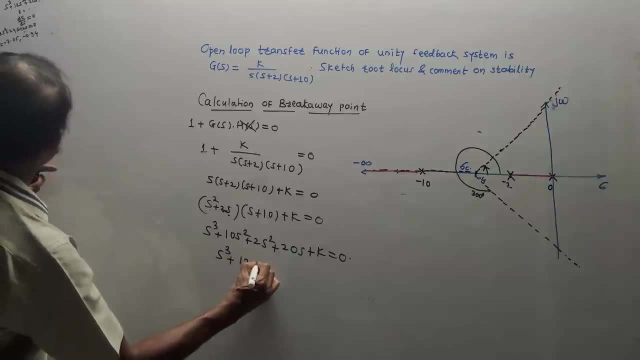 S cube plus 12 s square plus 20 s plus k is equal to 0.. We have to generate the equation of k with this, So I will write it over here: k is equal to. We will keep this k here. 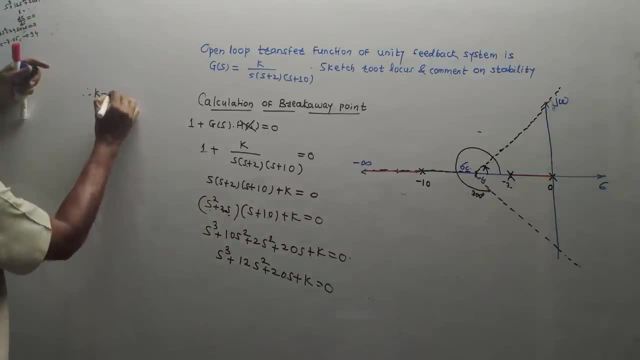 We will transfer the rest of the terms to RHS. So k becomes minus s cube, minus 12 s. square plus 20 s plus k is equal to 0.. 12 s square minus 20 s. This is the value of k. 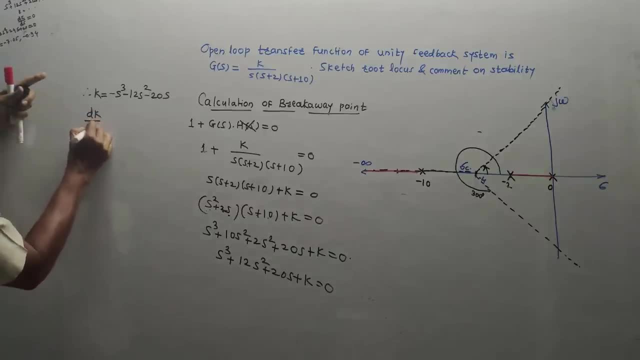 Now we have to take its derivative, That is, dk by ds is equal to. Its derivative will be minus 3 s square, minus 24 s, minus 20.. And this has to be equal to 0.. Therefore, I will write. 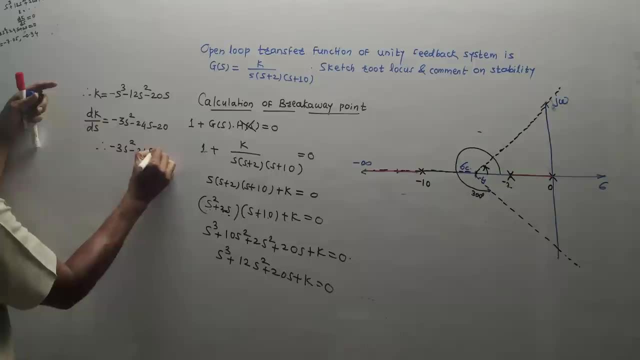 Minus 3 s square Minus 24 s minus 20 is equal to 0.. All these terms will be plus, because we are equating it to 0. So this term will be: 3 s square plus 24 s plus 20 is equal to 0.. 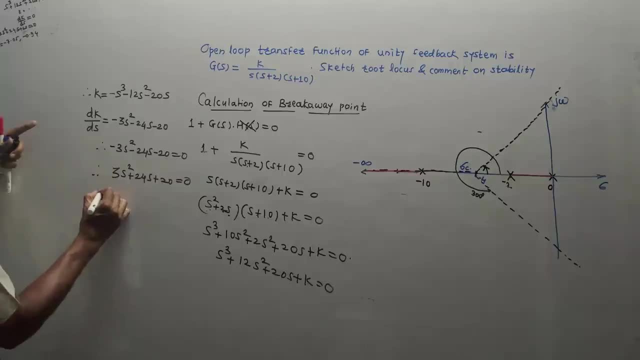 We have to calculate the roots of this on kelsey. So if you calculate the roots you will get answer of yes. One answer is minus 7.05.. Another answer of yes is minus 0.94.. That means two breakaway points have come. 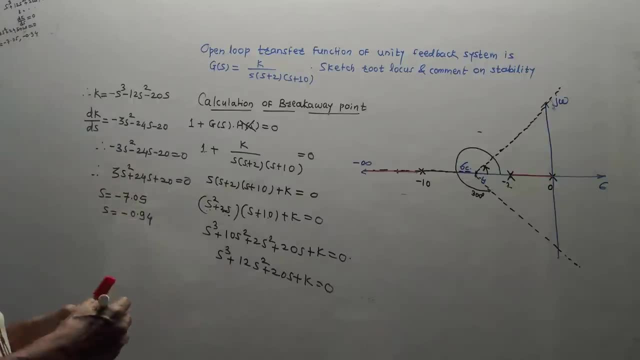 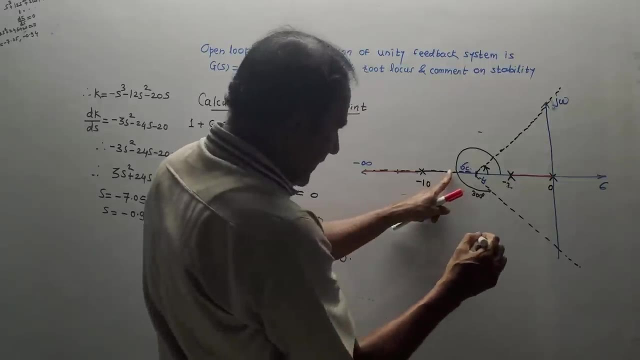 Now which one is valid from this? How to check this? It is a very simple technique: See minus 7.05.. This point it will be somewhere here. It is not part of root locus. How to remember: Two points have come. 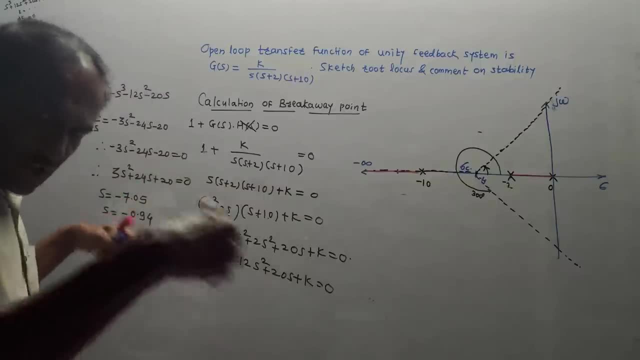 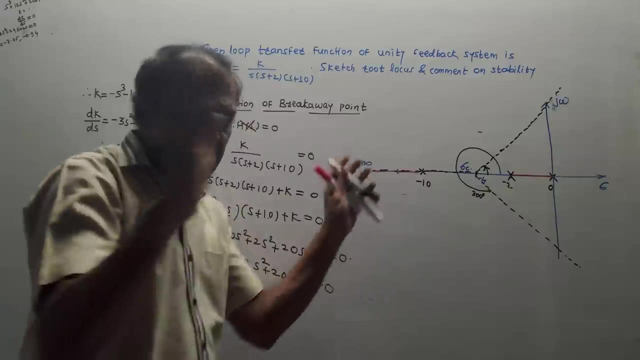 Which point is lying on the part of root locus? We have already highlighted In this diagram the reading I have made. that is part of root locus. So from this minus 7.05.. Is not the part of root locus? because I have not drawn from the reading. 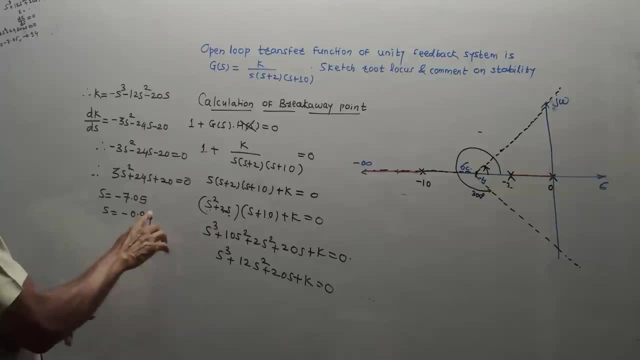 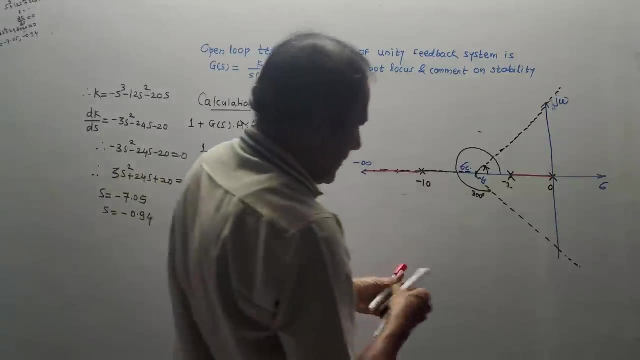 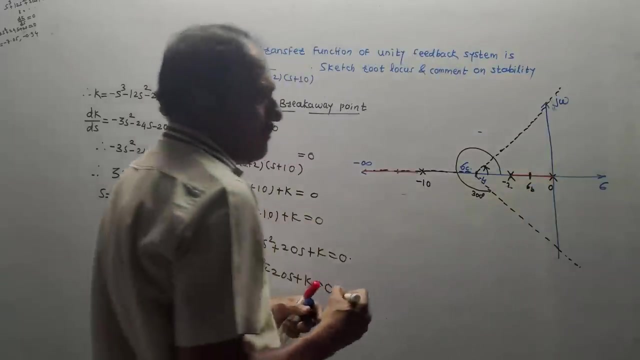 But minus 0.94 is part of root locus. So the part of root locus minus 0.94 means this value somewhere here. So this is the breakaway point. I will write it by sigma b, Any notation will do. 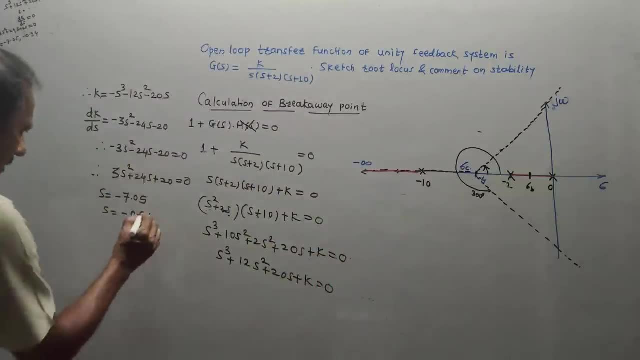 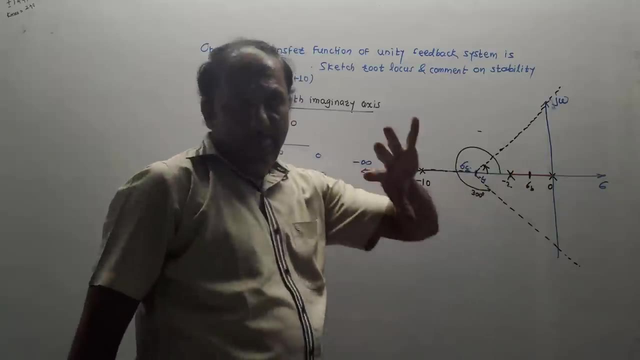 This is the valid breakaway point, which is minus 0.94.. Now next step. See, in this numerical there are no complex poles. So what we have written: angle of departure, angle of arrival, that is not necessary to be calculated. 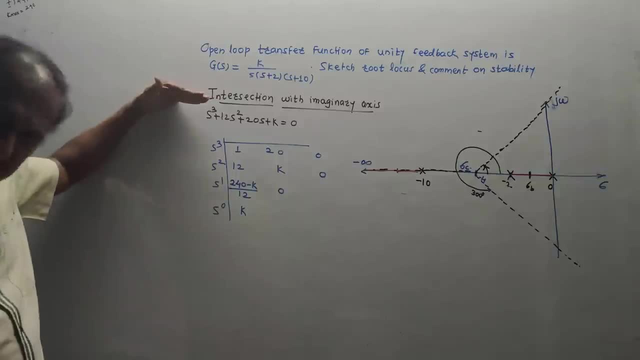 That step is not applicable, So I am directly writing. next step: Intersection with imaginary axis. We have prepared this equation. We have already done it in the last step. As it is, I have written And made a route array Just to show that I have already written the route array. 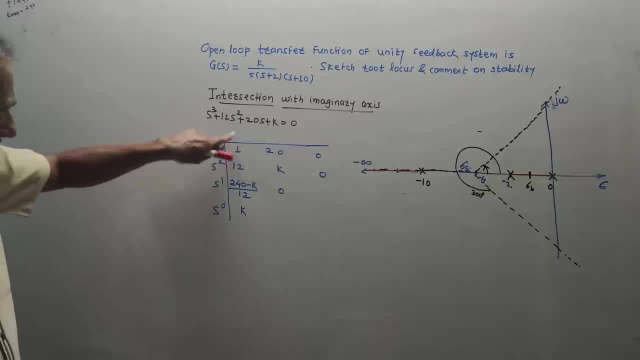 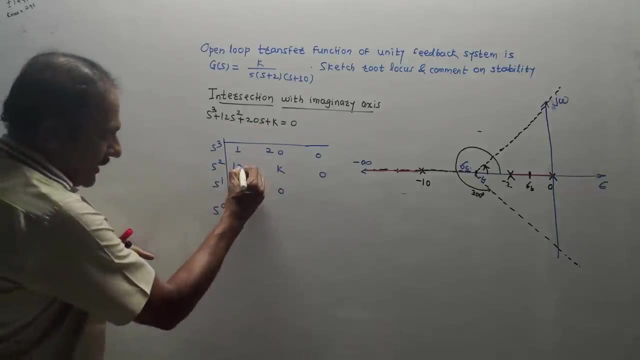 We know the procedure: how to write the route array. This is coefficient 1.. Alternate is 20.. Next is nothing, So 0. Then second coefficient is 12.. Then this is k. Then how to calculate this? 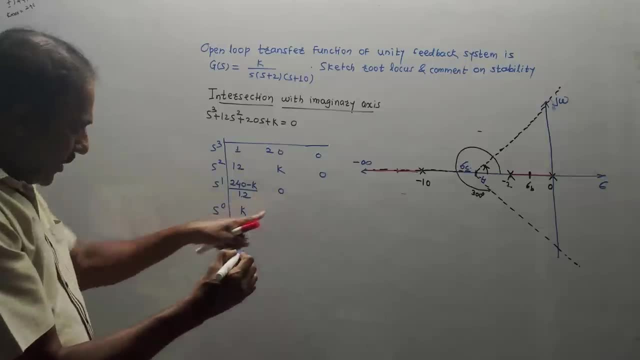 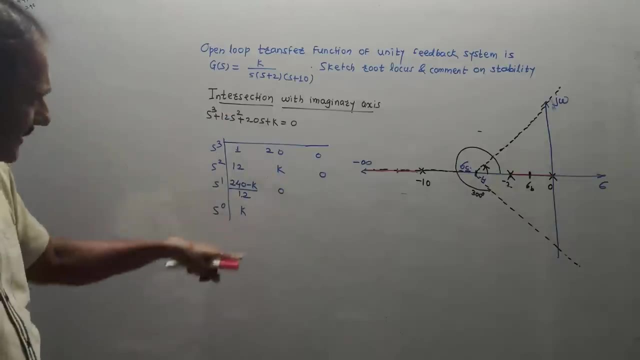 12 into 20 minus 1 into k upon 12.. This will be 0.. How to calculate this? This into this minus 0 divided by this. If we do this, then this answer will be k. So this is the route array. 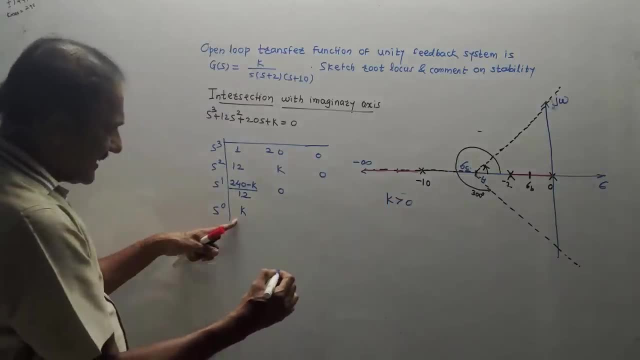 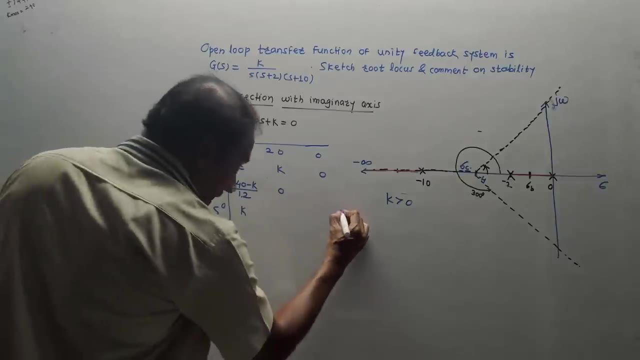 We know for stability, k should be greater than 0. from this And this it should be also greater than 0. So likewise we can calculate the stability. But we are interested, We are interested in calculating value of k marginal. 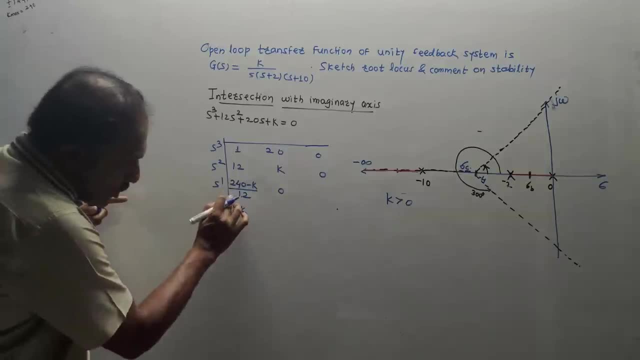 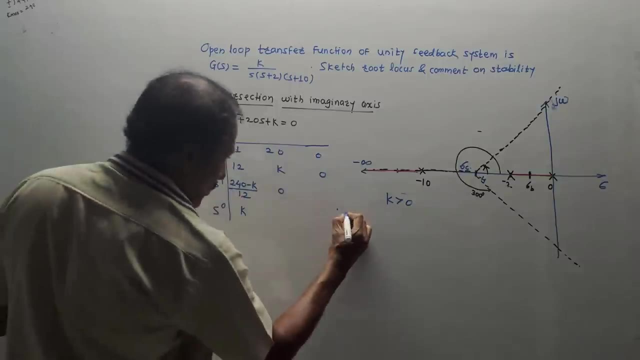 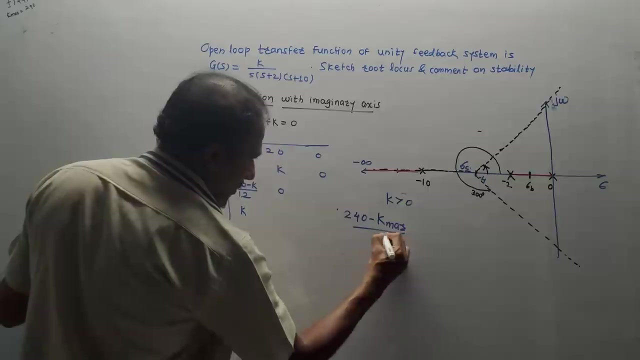 See, For marginal stability we should have any one row that should contain all 0s, So one is already 0.. So we have to make this also 0.. So for marginal stability we can write: 240 minus k, marginal upon 12 is equal to 0.. 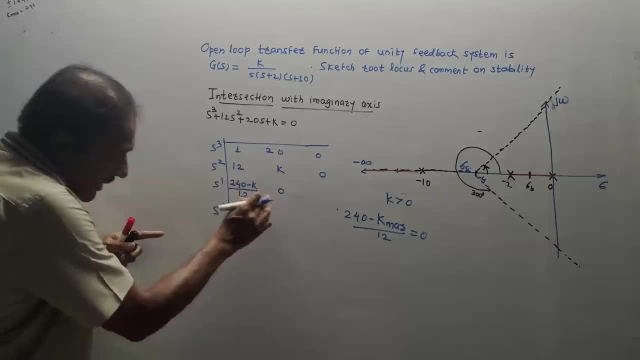 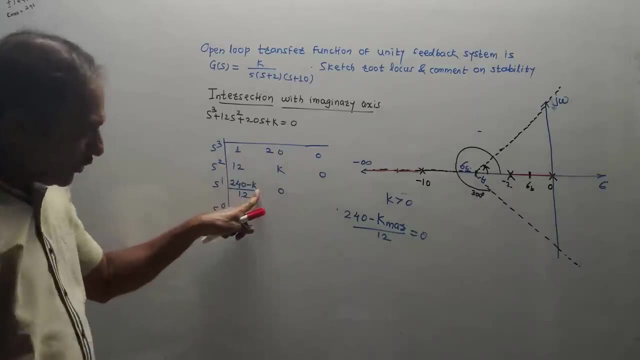 We have already solved this type of numerical. So see, We need a whole row in which all 0s should be there. This is 0.. To make this 0, we have to make k's notation k marginal. This is called marginal stability. 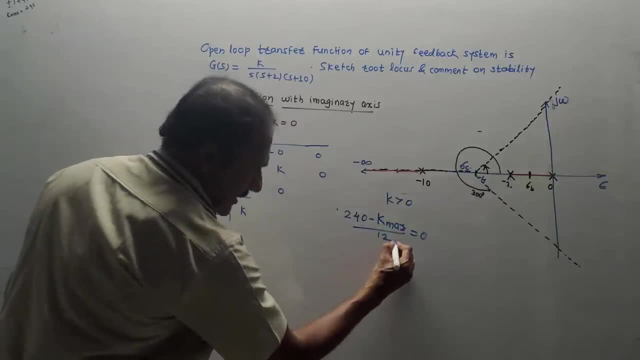 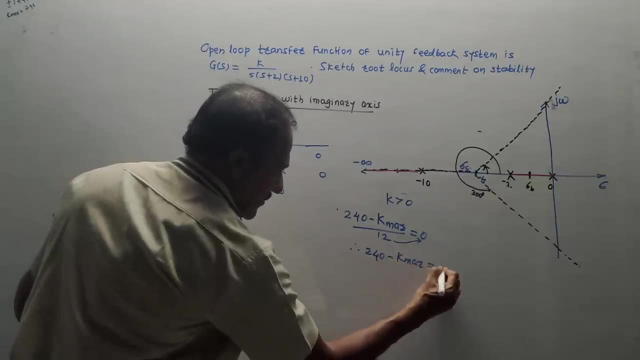 Now we have to calculate the value of k marginal by this. If we transfer 12 here, then it will become 0.. So I will get 240 minus k marginal is equal to 0. Simple logic. If we transfer k marginal here, then I write: k marginal is equal to 240. 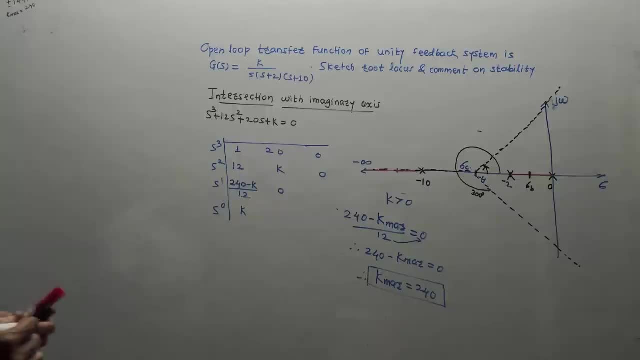 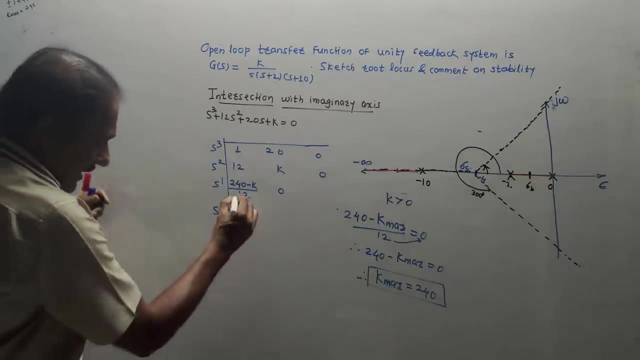 So marginal value of k is 240 degrees. Now what is the rule? Take this value. We have to take this value and make an auxiliary equation Means we have to consider the equation before this. So auxiliary equation, which is AE: 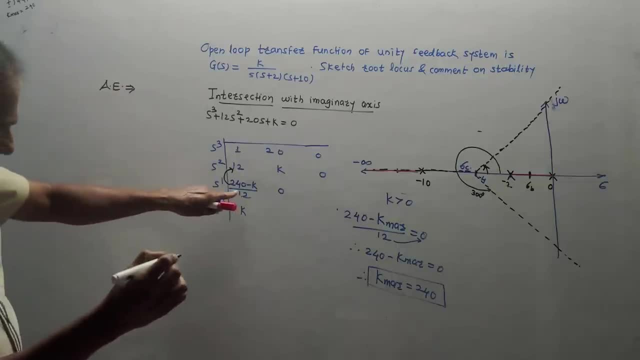 Auxiliary equation can be written as We have to use this value and see the equation above this. So it is 12 into s square. This is the row of s square. So I write like this: 12 s square. We know that there are alternate elements. 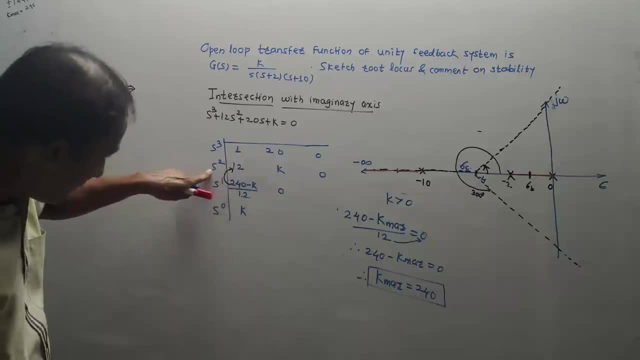 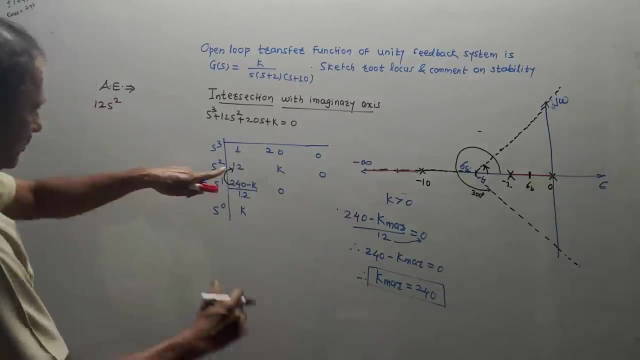 Means, if this is the term of s square, How did I write s square 12 into this term S square? Then s will not come. After that constant will come, Because every row contains alternate terms. So equation is simple. 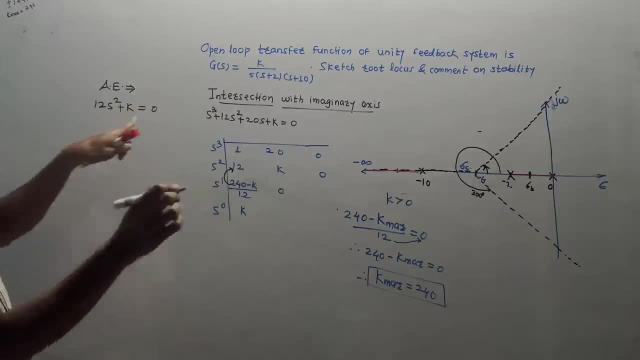 12 s square plus k is equal to 0.. K means by default k marginal in this case, Which is this value. So I write this equation like this: 12 s square is equals to plus 240.. Value of k and k marginal is equal to 0.. 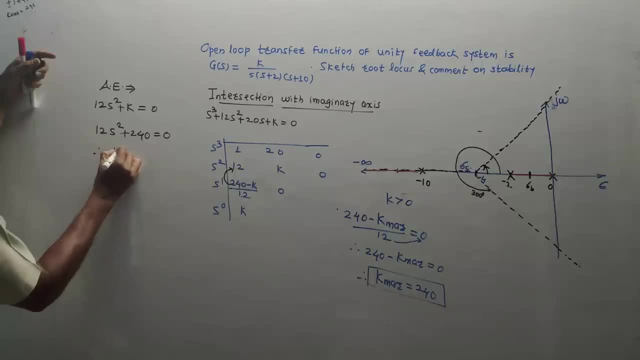 Therefore, this will come: 12 s square is equals to minus 240.. Therefore, s square is equals to minus 20.. I will just transfer this to another set, So 240 upon 12. It is minus 20.. 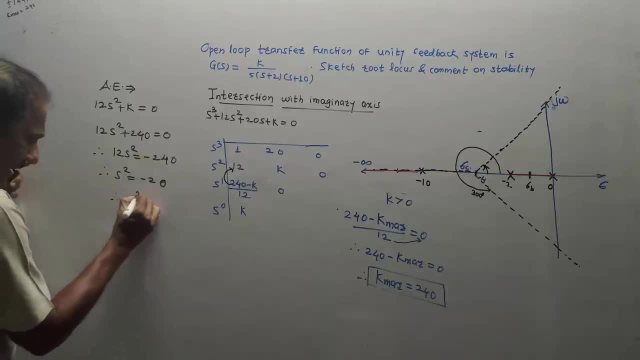 We have studied these types of numericals. As you can see, we write like this: Whenever minus sign is coming, we write j square And 20, as it is Means for minus sign. I have written j square And 20 as it is. 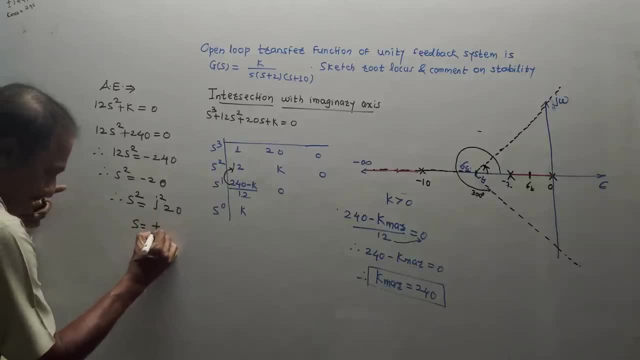 We have to get its square root. So take square root. To write square root we have to write plus, minus. Square root of j square will be j And root 20 has to be solved on calc, So it is 4.472.. 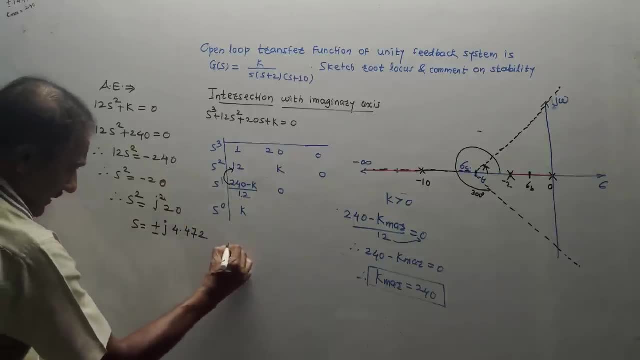 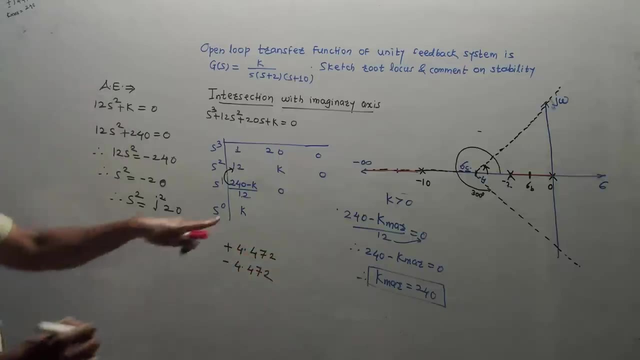 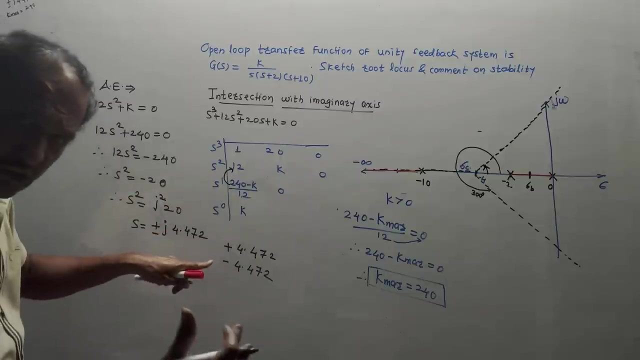 This value has come. One value is plus 4.472.. And the other value is minus 4.472.. These are the points at which the asymptotes crosses or touch to the imaginary axis. So we have to mark this point. 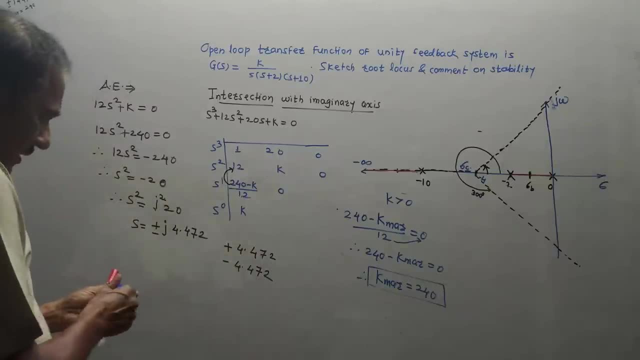 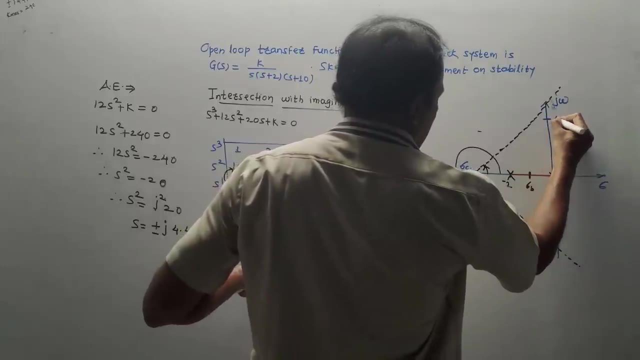 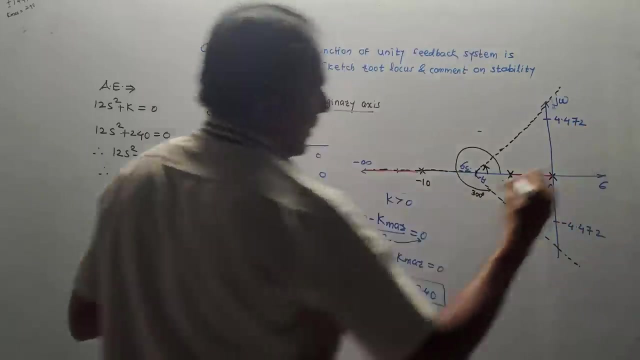 Means this point is minus. The first point is plus 4.472.. So somewhere here I will write Plus 4.472.. And the other is minus 4.472.. These are the points at which root locus, not asymptotes. 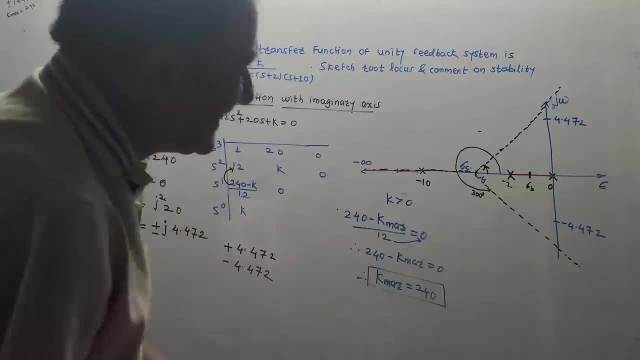 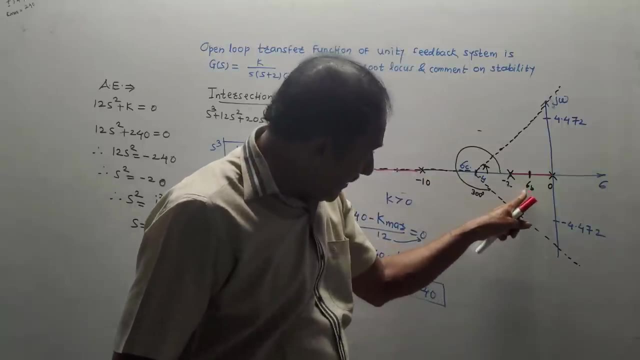 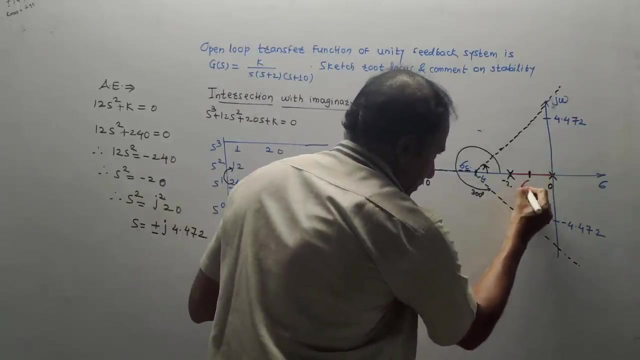 root locus touches to the imaginary axis Which I have marked. Now the last step. We have already marked the breakaway point of sigma b, So from this point, this point of sigma b, I will use another color. This is the breakaway point of sigma b. 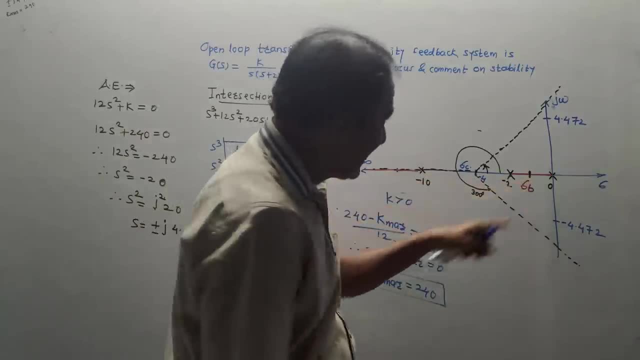 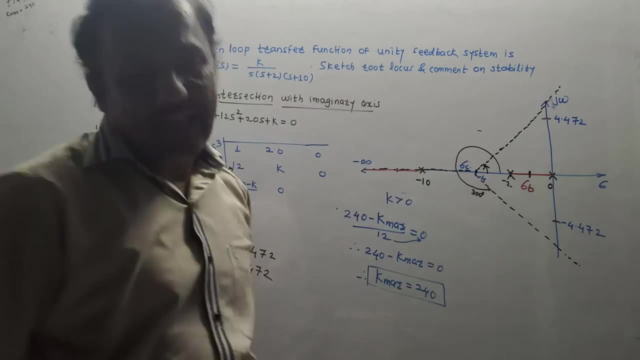 Which is minus 0.94.. We have already marked this. We have marked the points of intersection. So the last step is to draw a curve, And one rule is that root locus is always symmetric about real axis Means. the curve will be like this: 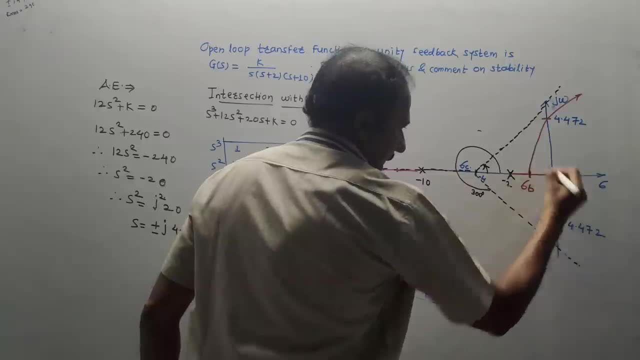 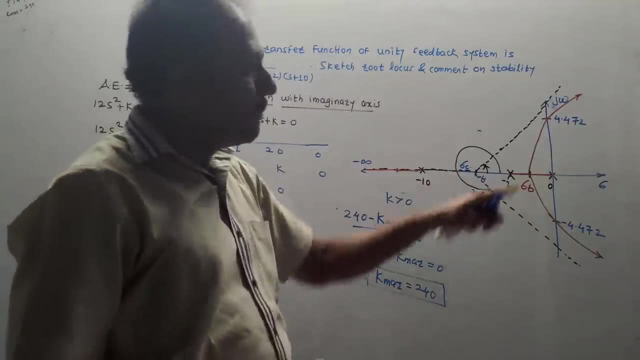 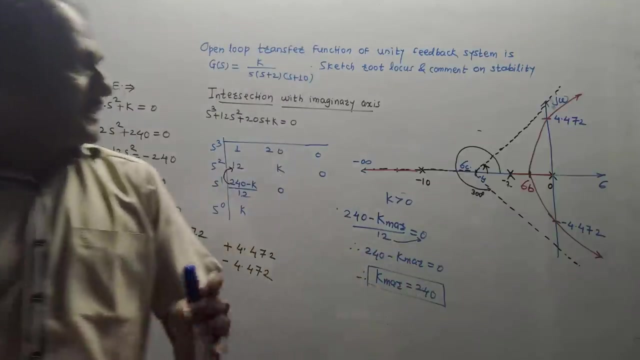 This type of curve towards infinity. And second point is this point like this: This is towards infinity. So this is the complete root locus. So, dear students, That's it for today's session, Thank you. Thanks a lot for watching this video. 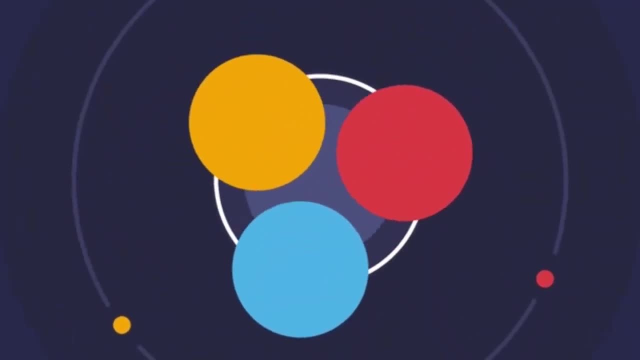 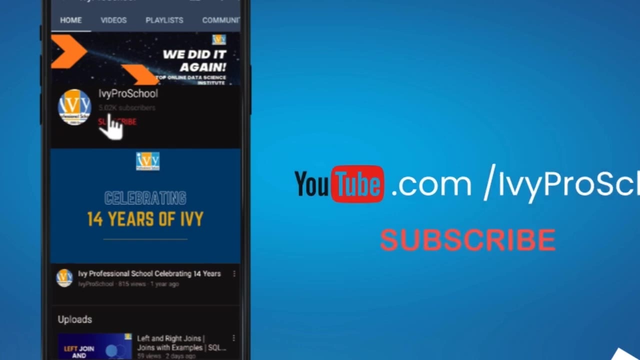 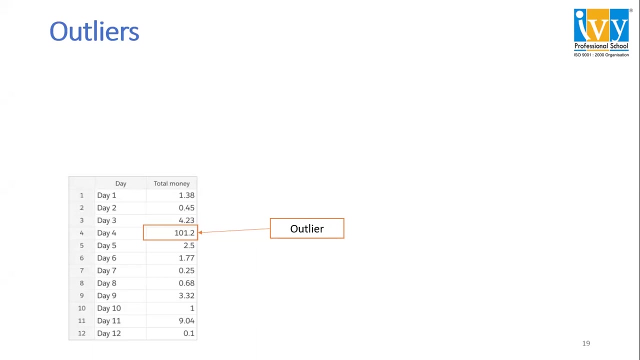 Hello everyone, Welcome back to Ivy's YouTube channel. We are back with another video on the data cleaning series. Our today's topic is going to be outliers. Data points that are significantly different from other data points are called outliers. Outliers can skew the 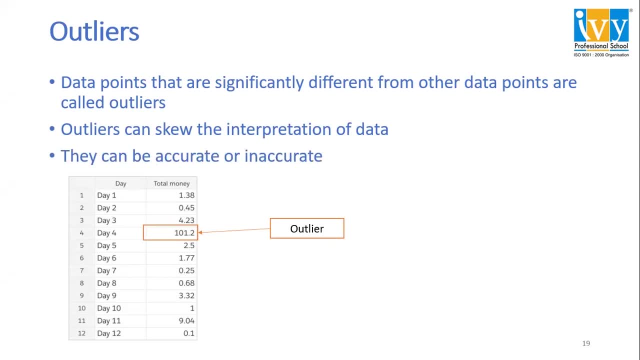 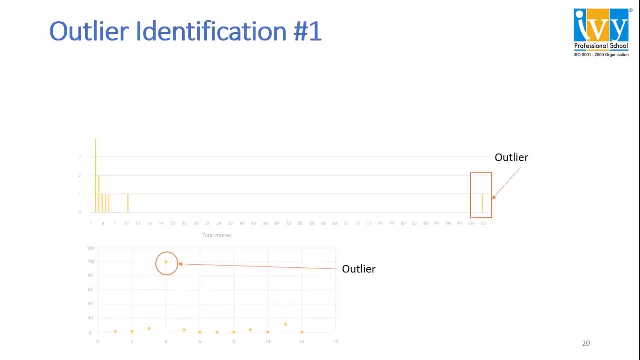 interpretation of the data. They can be accurate or inaccurate. Let's have a look at the first method of detecting outliers, The outlier identification one. Here we see there are two types of charts. It's a visualization which has charts like histogram and scatter chart with